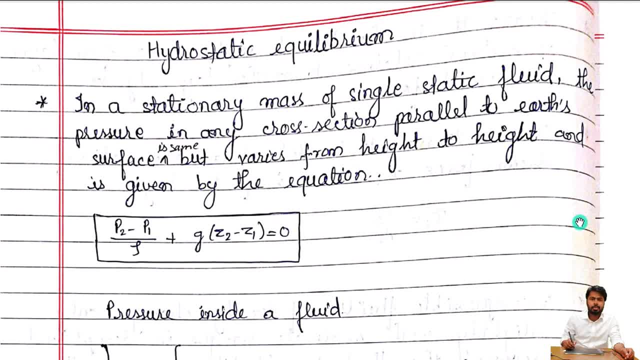 what is hardware static equilibrium? so a fluid is said to be, in hardware, static equilibrium when fluid is at rest or in other. in other words, you can say as when? when the fluid velocity at each point is constant over time. okay, when fluid velocity at each point is constant over. 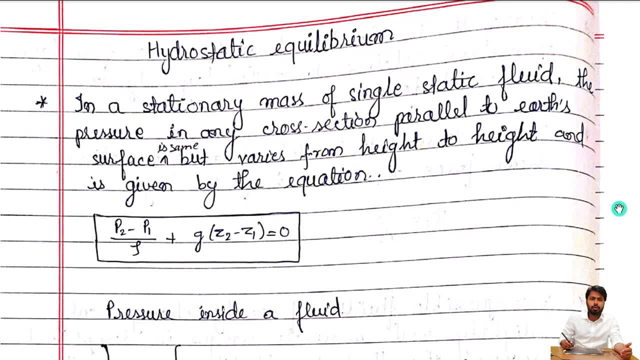 time, then at that condition we can say as fluid at rest, and okay, this is. this situation is called as hardware static equilibrium. so let's see, so you can see it here: in a stationary mass of single static fluid, the pressure in any cross section parallel to the earth's surface is same but varies from height to height and is given. 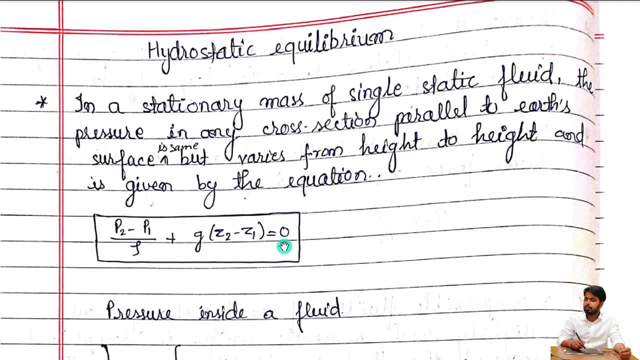 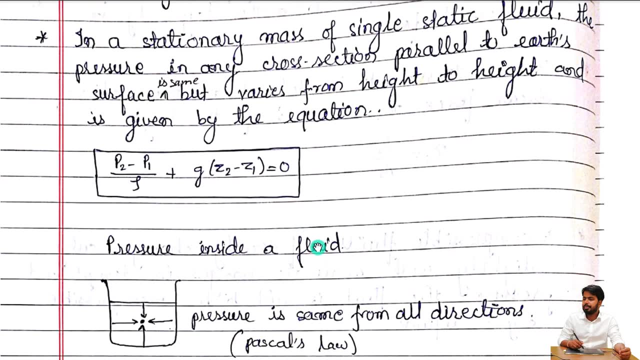 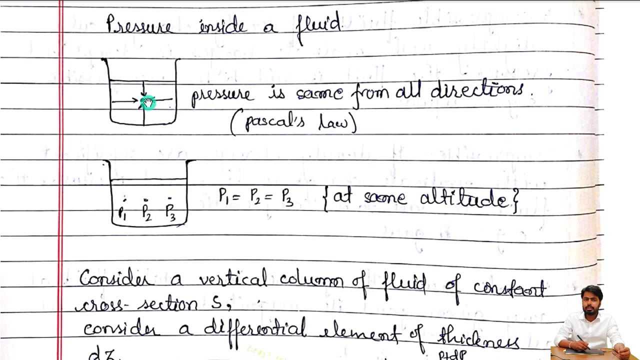 by the equation p2 minus p1, by rho plus gz2 minus z1, is equal to zero. so any fluid, okay, static fluid- which will follow this relation. what is that hardware? static equilibrium glass. on this one, however, right up the plane, precept inside of flood, okay, suppose. 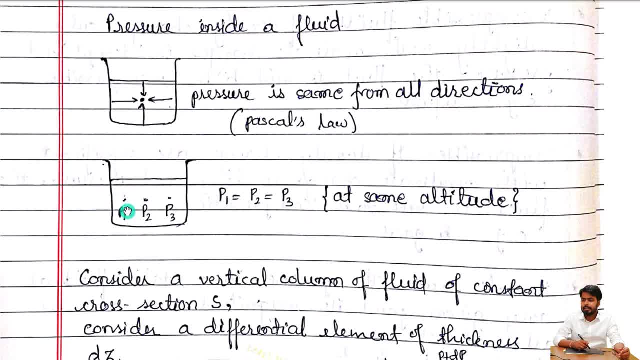 so here, P1 is equal to P2 is equal to P3. if all these are in the same level, then the pressure will be the same at the same altitude in gate, I guess in 2011 or something. one question was asked: this type of shape was given. then again, this shape was given. then again, this shape was given. 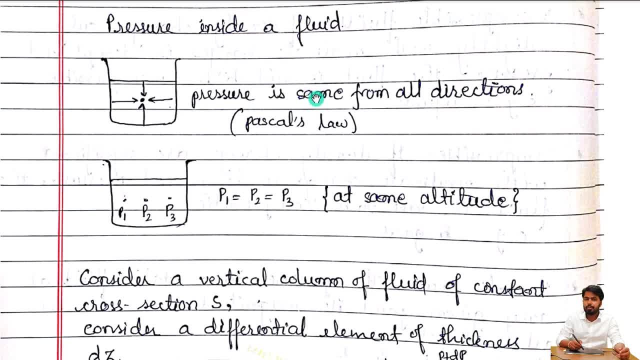 and at the height of all three at different point means P1, P2, P3 was given. in that case you were given four options. when P1 is equal to P2 is equal to P3 and P1 is greater than P2 is equal to P3. 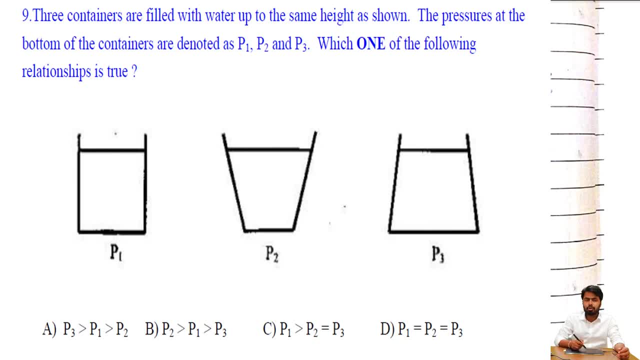 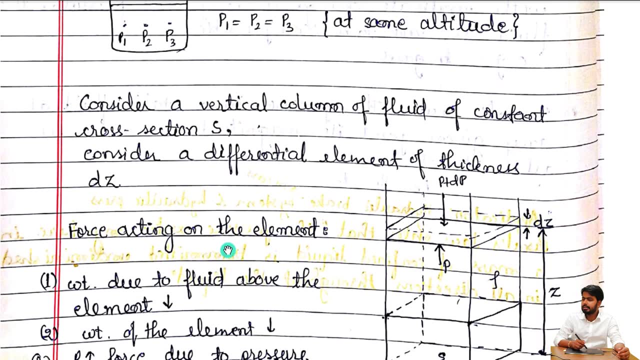 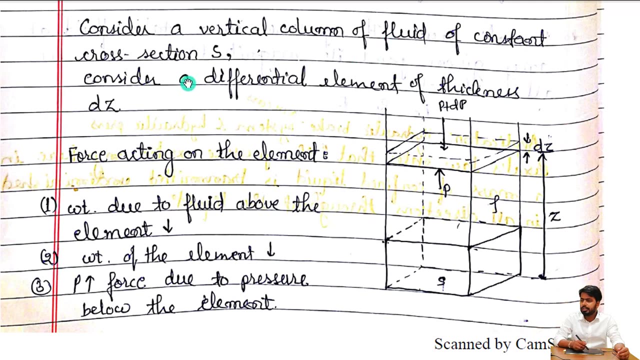 these four options were given. so what will happen? in that P1 is equal to P2 is equal to P3, option was correct. I will check that question. ok, now let's see. let's do the force balance, ok, so consider a vertical column of fluid of constant cross section S. 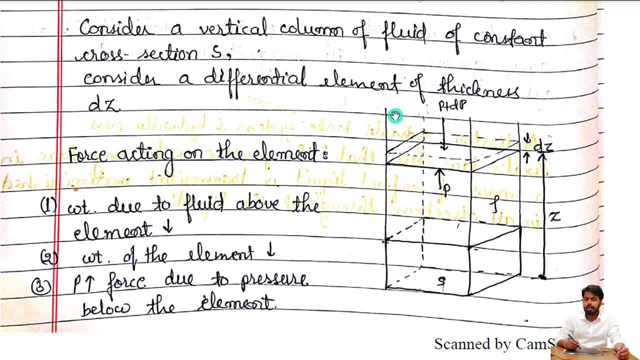 consider a differential element of thickness. dz means a hydrostatic equilibrium. ok, this is our cubicle in which we will balance the hydrostatic equilibrium, right, so let's take one element in it. this is called dz. let's take one element on which we will do hydrostatic equilibrium. 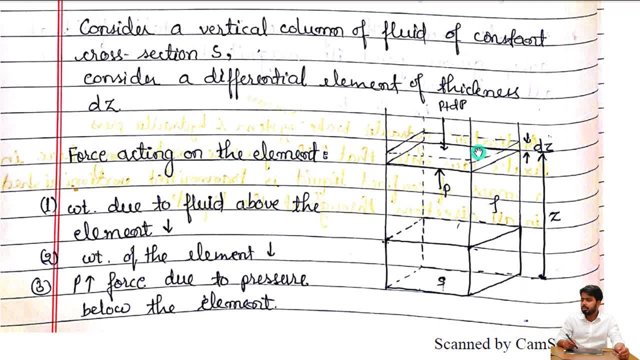 and we will extend it later till z. ok, so this cross section is like this: fluid density is rho, P is the pressure from the bottom side, P plus dp. pressure means from the upside, element, cap. ok. so which force is applied on this element, let's see first, then we will do the force balance right. 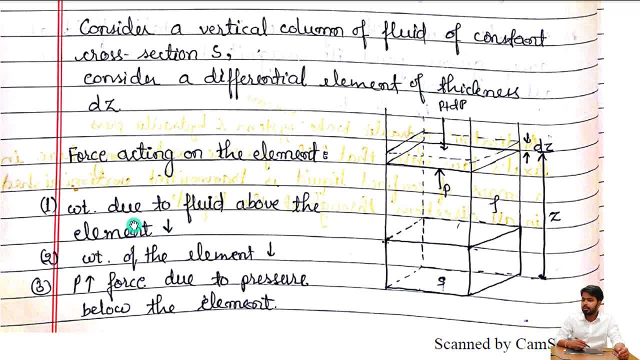 so force acting on the element. so first, force is weight due to fluid above the element means the weight of the element, the force applied on it. ok, weight because of the weight. so what will be the weight? P plus dp? force applied into the cross section area. so the force will come right. 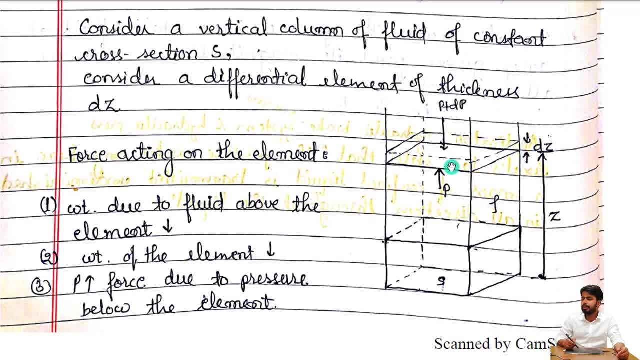 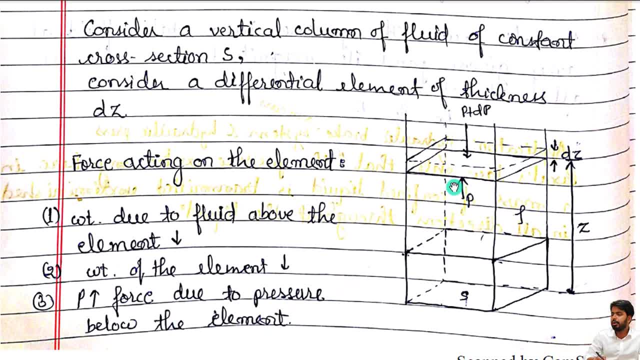 now weight of the element. weight of the dz element will also work in downward direction. third, P force due to pressure below the element. so the pressure will be applied in upward direction because it is applied from the bottom. so it will be applied in the opposite direction and the force above P plus dp. 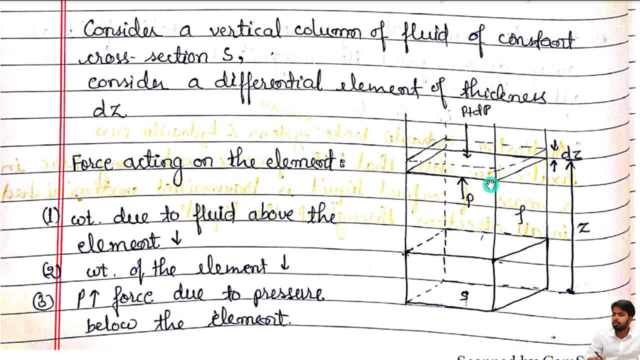 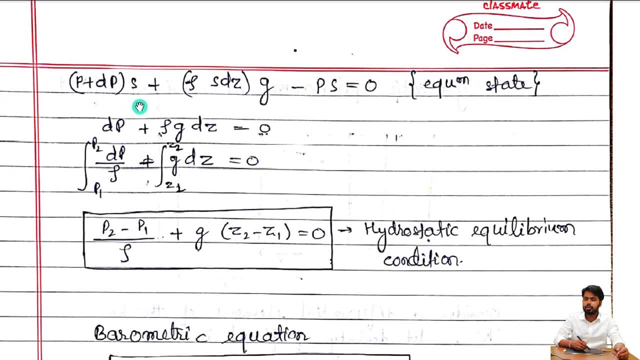 which is up fluid element, and weight of the element. these two will work in downward direction, means they will act. now we will do the force balance. so first P plus dp into s cross section is done. now weight- what is weight mass? into gravitational force, mg. so rho density is done. 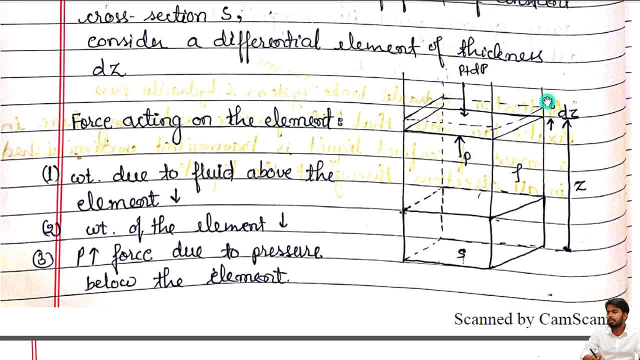 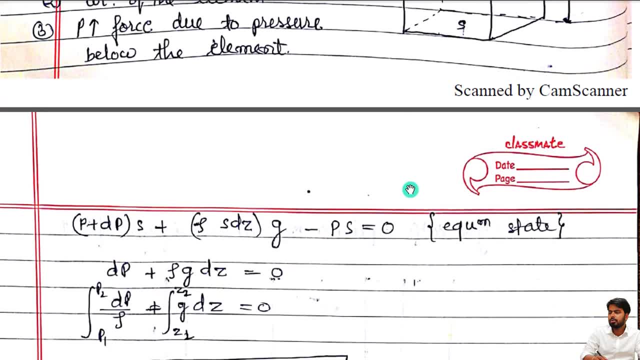 what is s into dz. your volume is done. cross section area is s, so dz. cross section area into that height means what is your volume, so what is the volume of this element? and density is rho, so mass is done, so rho s dz into g. what is this? 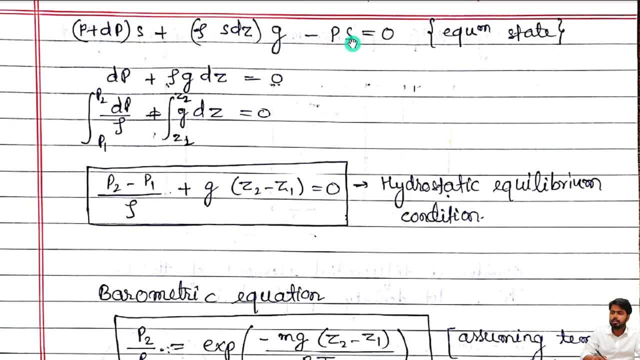 mass is done into g minus P, s pressure is from the bottom side and this is cross section area. now we will exist this in equilibrium state condition. so if we solve this, we will find that dp plus rho g dz is equal to zero. so dp by rho plus 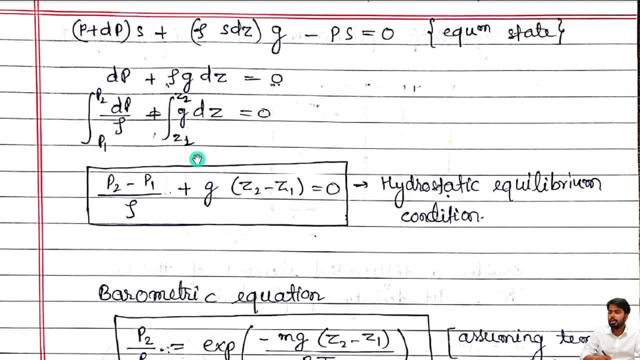 g, dz is equal to zero. now if we integrate z1 to z2 point, z1 to z2, so at one point P1 will be P2. so P2 minus P1 by rho plus g, z2 minus z1 is equal to zero. so this is hydrostatic equilibrium condition. 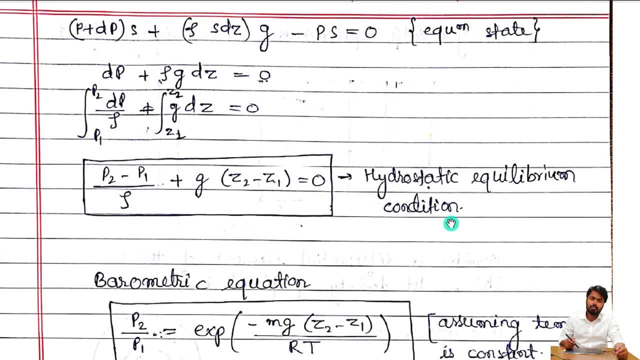 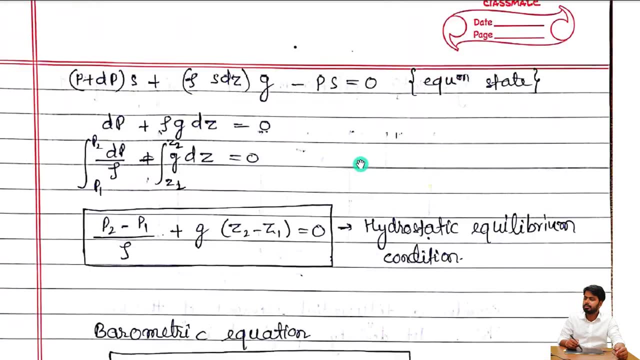 means any fluid is in rest condition and in hydrostatic equilibrium condition it will follow this relation. so this is your hydrostatic equilibrium condition. this is a question which I have asked earlier. first time we have discussed this is its derivation. ok, now we will move to the barometric equation. 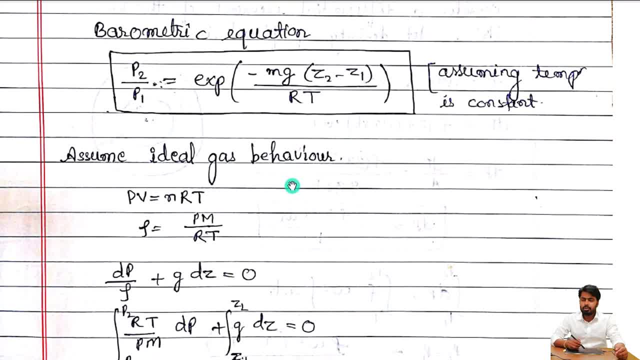 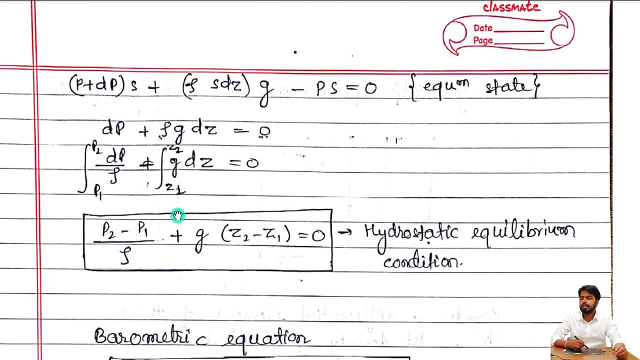 what is in barometric equation if we assume for ideal gas, if we do balance of hydrostatic. so what happens here? in liquid case, density is generally constant. what is density we have taken constant in time of integration. but if it is air? so what happens with pressure? 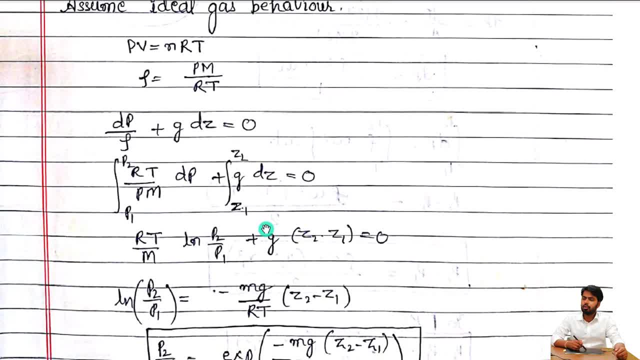 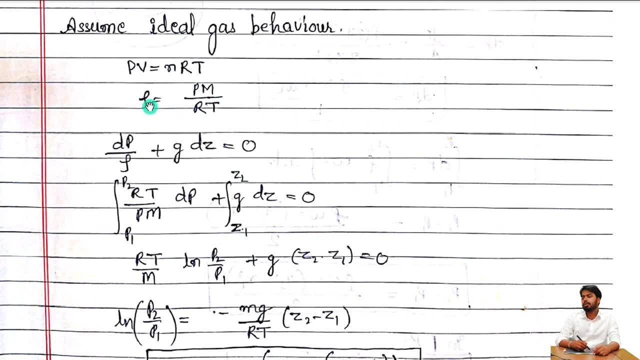 its density changes. so we need to account that also. so here we will take the accountability of density also. ok, we can't take as constant. so PV is equal to nRT, so rho is equal to what will happen. PM by RT will come here. you calculate and what. 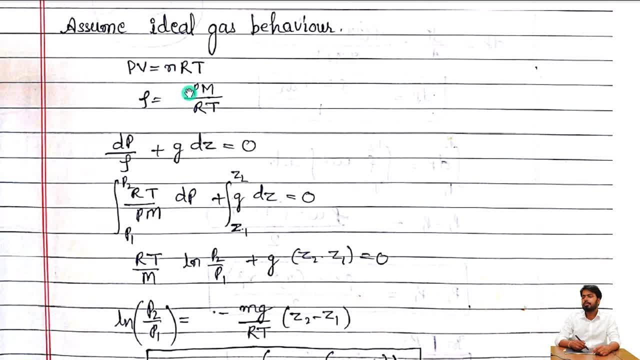 number of moles is equal to what was weight by molecular weight. so weight divided by V density will come and this molecular weight will be divided. so PM divided by RT is equal to what will come: rho, so rho is equal to PM by RT. so DP by rho plus. 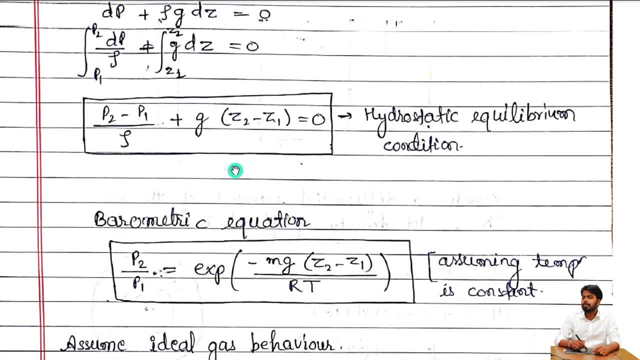 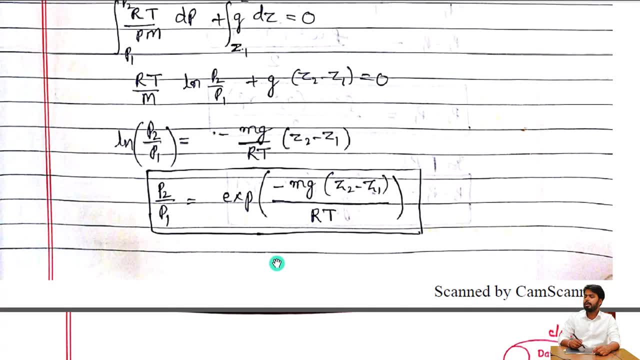 g, dz is equal to zero. so this relation which you have here, what is in this? instead of rho, we will put PM by RT value. ok, so PM by RT. now we will integrate this, so final value will come. this will come, this relation will come. P2 by P1 is equal to. 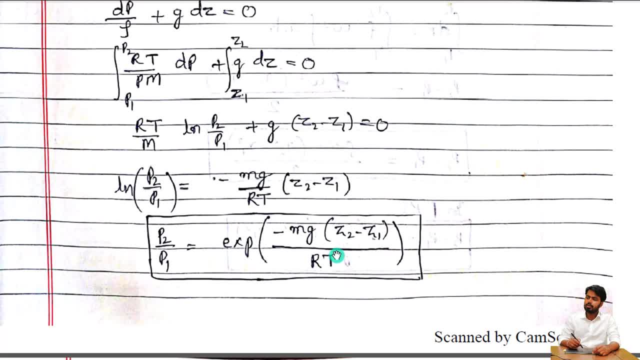 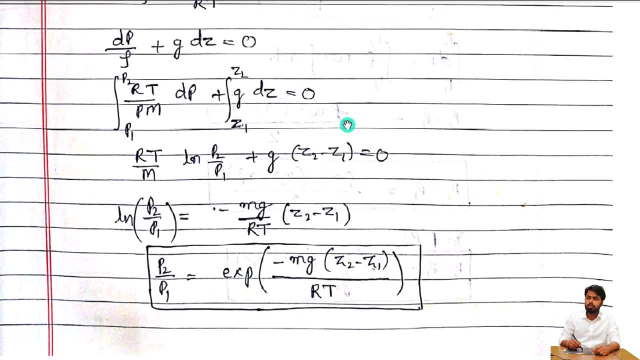 exponential minus mg, z2 minus z1 divided by RT. so this is the equation. please do remember this formula. ok, P2 minus P1 is equal to exponential minus mg by RT into z2 minus z1. so this relation is very, very important sometimes in GATE. 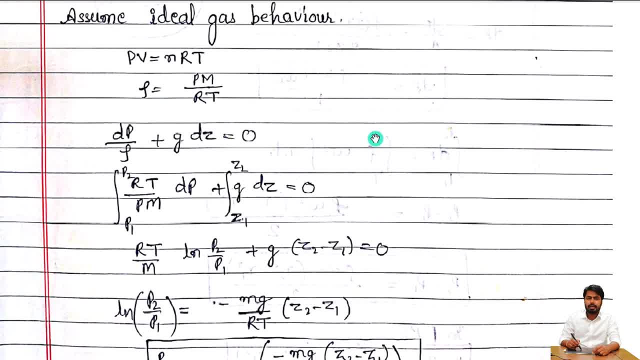 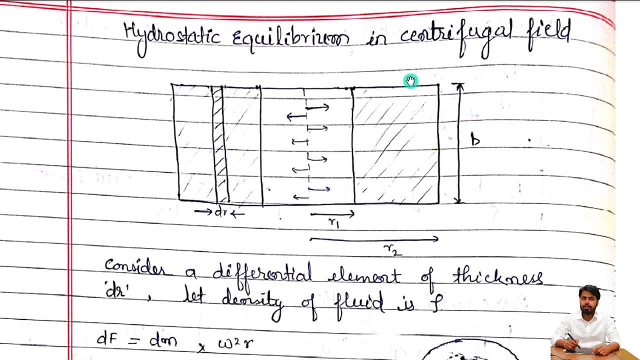 sir, direct question has been asked one or two times. ok, now we will see here how to stack equilibrium. second, how to stack equilibrium in centrifugal field means in this case how to stack equilibrium, because here the fluid will rotate, but if the rotating fluid its velocity at each point. 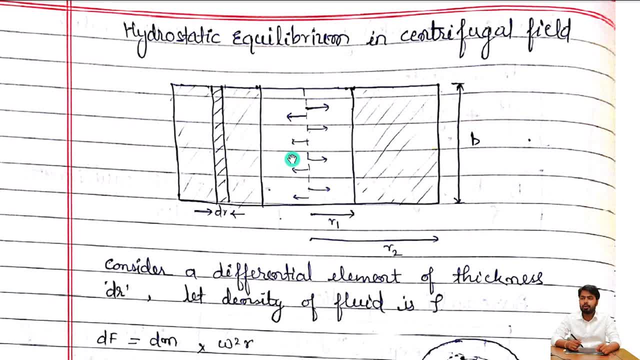 will be constant over the time. ok, so in that case, how to stack? equilibrium can exist in centrifugal field, and that centrifugal force actually will balance it. so let's see here what is this your front view. if you take any vessel, then what is it front view? 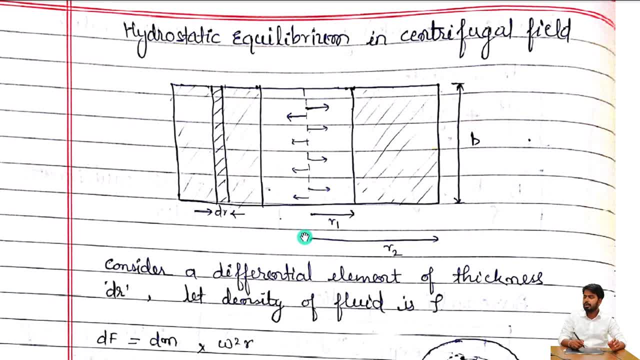 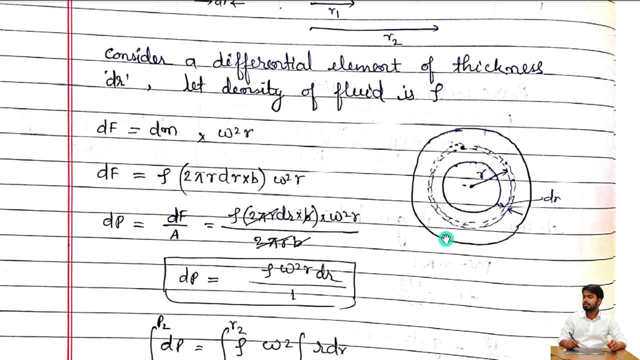 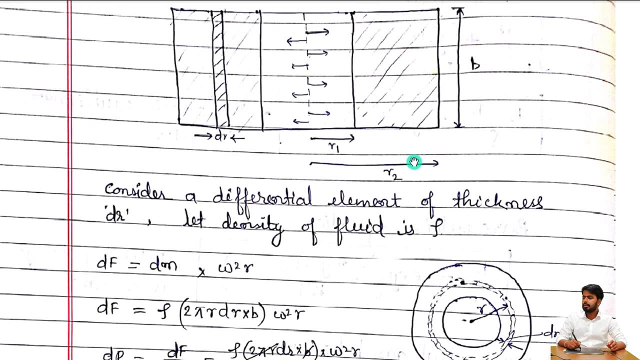 and it is- is a fluid. ok, now we will see. here, sir, we have concentration of this and in this, here, if we have some flow along the surface and we have the strength and the fluid in terms of omega. so what is omega? angular velocity in terms of acceleration: what is angular acceleration? omega square into r. 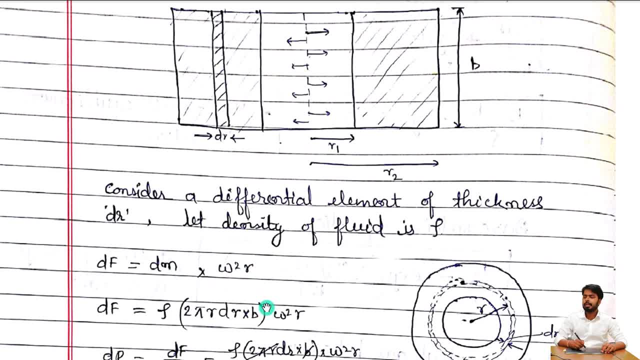 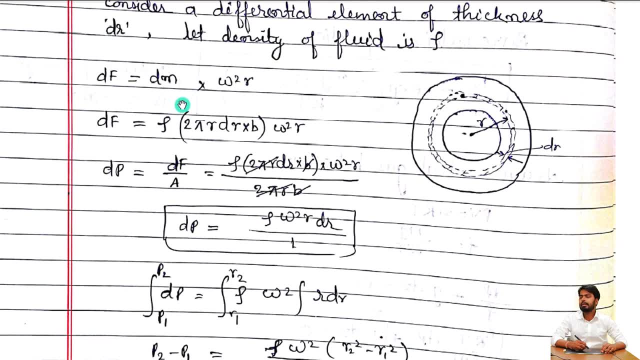 so force equal to dm into omega, square, into r. now, what is dm? how will you find dm? now, to find dm, what will be dm? density into volume, correct. so density, how will you find volume? suppose this is r radius, so this is dr. so what will you do? pi? r plus dr, whole square. 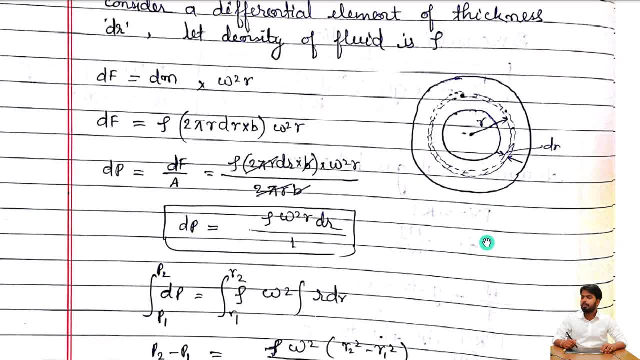 minus pi r square. if you do this, you will find that your net area change is 2 pi r dr, correct. so 2 pi r dr will come. we can neglect the square of dr. so if 2 pi r dr will come, what will be? that area will be into width. 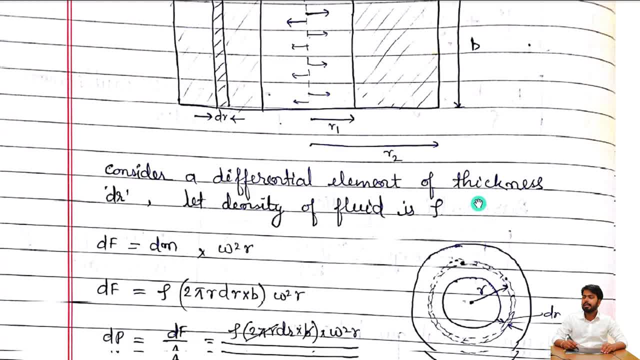 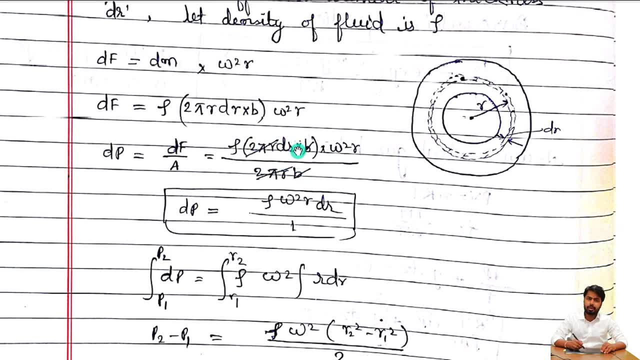 so what will be our width? this will be width b, so 2 pi r dr into b, so our area will come. 2 pi r dr into volume will come into density, so our mass will come into omega, square into r. now dp is equal to df by a. what is cross section area? 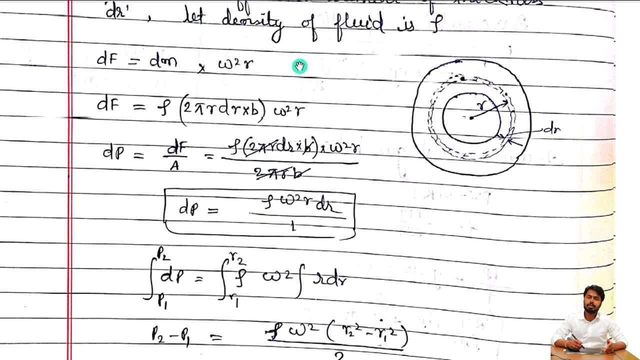 so what is cross section area? 2 pi rh is there? so 2 pi r. you know you can take length of b, so 2 pi r into b, this will be cut and dp is equal to rho omega square r into dr. 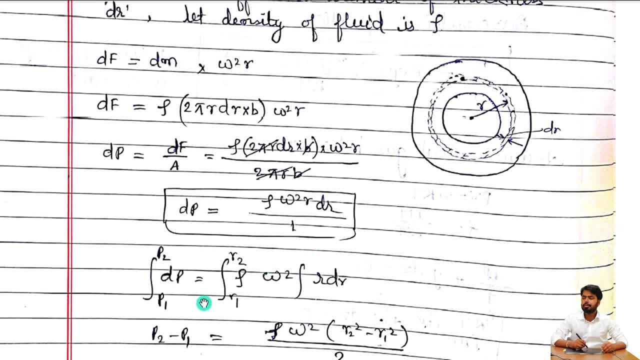 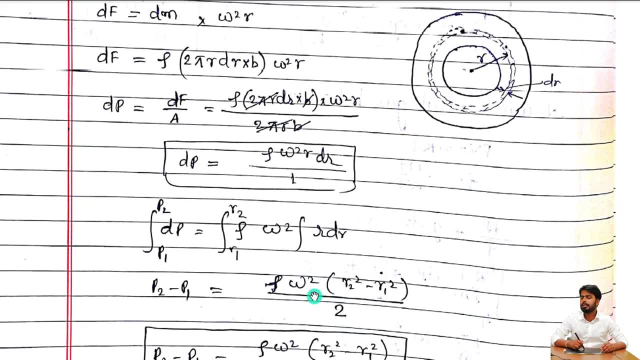 now, if you are going to integrate with respect to p1 to p2 dp, here you have to integrate from r1 to r2 as a integration limit. so if you are going to integrate, you will find that delta p value okay. p2 minus p1 is equal to rho omega square. 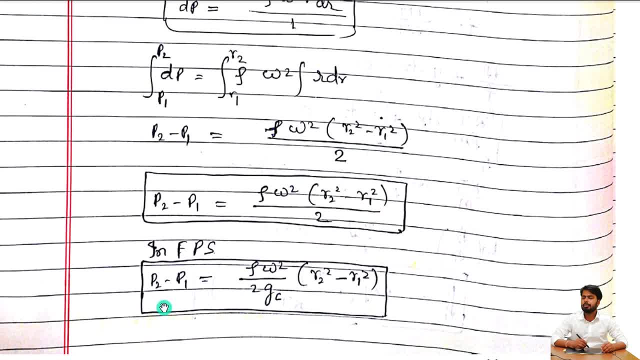 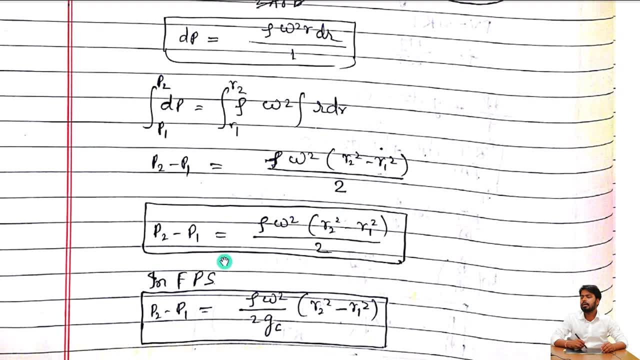 r2 square minus r1 square divided by 2, in fps system p2 minus p1 is equal to rho omega square divided by 2gc into r2 square minus r1 square. so this is the relation for hydrostatic equilibrium. centrifugal field means: 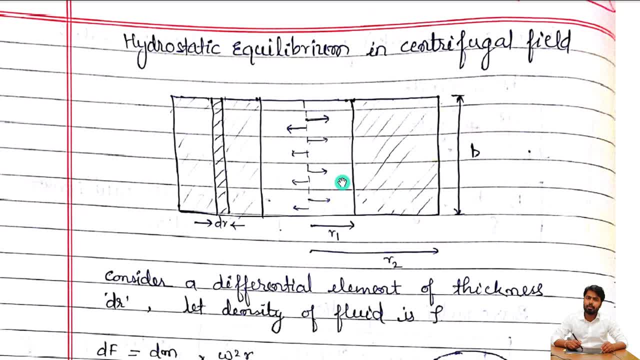 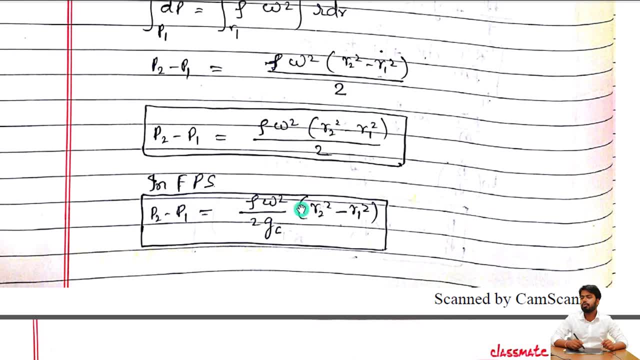 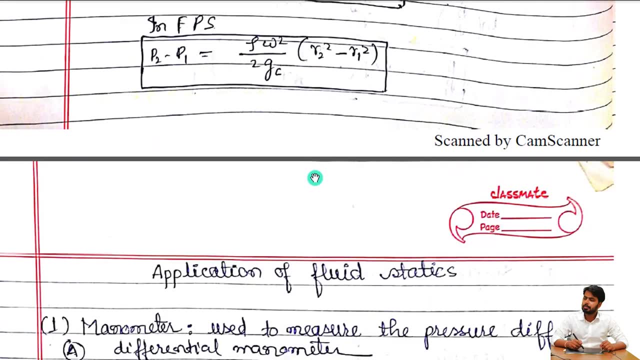 any fluid on the centrifugal field in hydrostatic equilibrium condition will happen only when it will follow this relation. so you have 3 derivations in the fluid statics. okay, now application of fluid statics. for this you will see 3 applications. first is manometer. 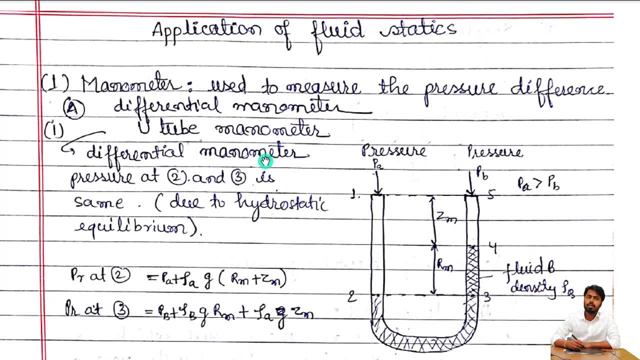 manometer is used to measure the pressure difference. what is manometer? it is designed to use? it is designed to measure the delta p- okay, change in pressure, and later sometimes they calibrate it in flow and use it in flow meter also. so this is also used in differential manometer. 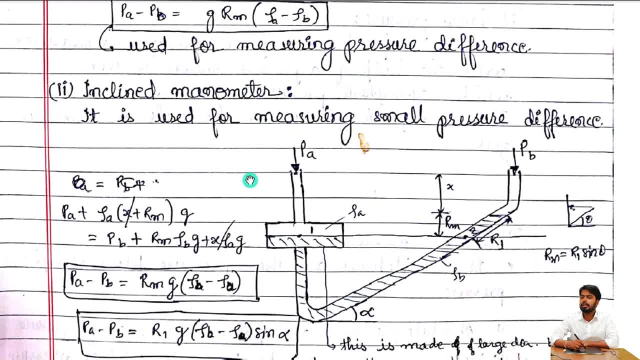 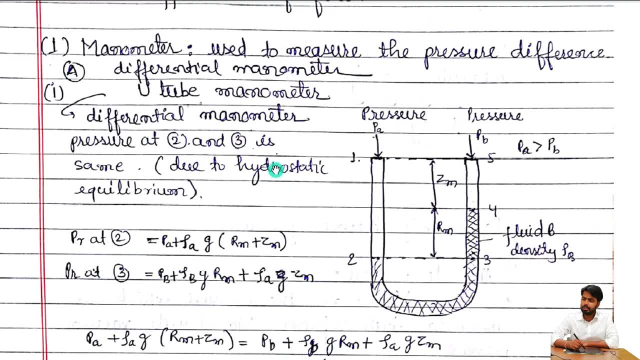 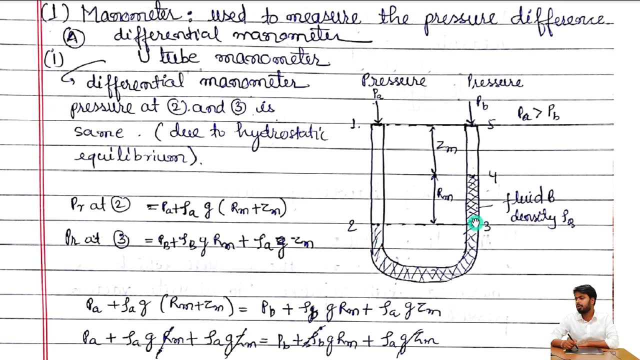 in differential manometer you get u2 manometer and in incline manometer, right. so what we do first is we will see u2 manometer. okay, so this is a simple setup of u2 manometer. okay, one fluid is this. what is the fluid of 0.2 to 0.3 point? 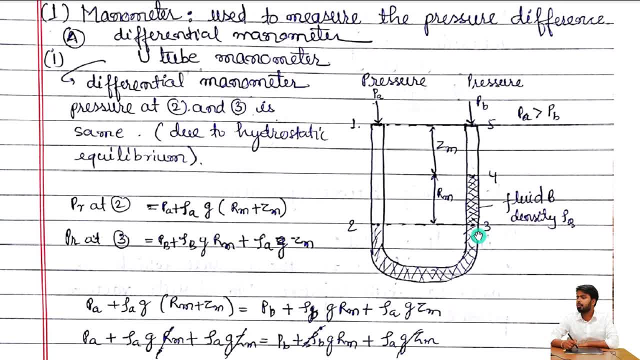 this is the fluid. second, what is your fluid? rho a, what is the fluid of this? this is rho a and what is the density of this rho v? correct now, first of all, what we have to do in this hydrostatic. 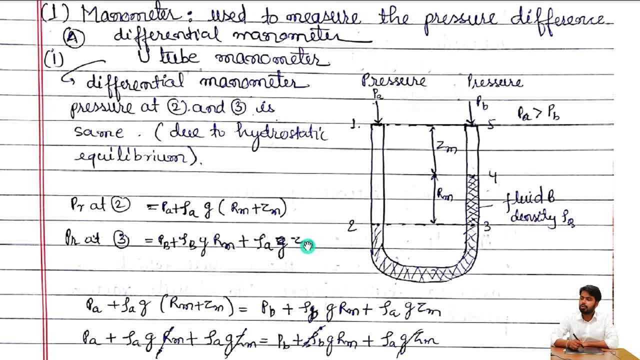 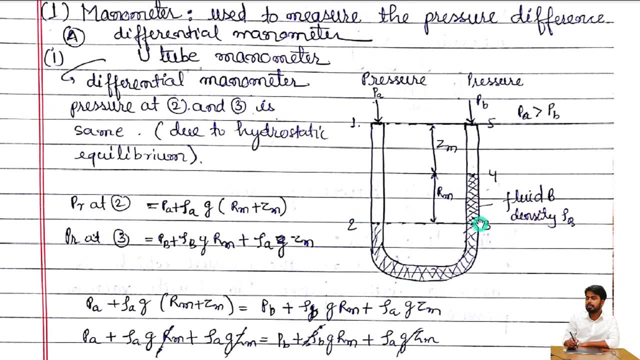 what is it? we have to balance it, okay. so, first of all, what we have to do is we have to draw a bottom line of pressure from where both of them draw a straight line of 2 and 3, from where, below that, there is no variation of density. 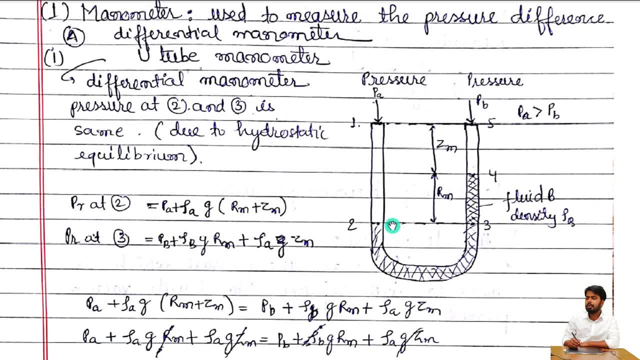 any numerical type. so draw a straight line from where the minimum level, where there is no variation of density and it is same fluid. so we will do it here. so this line will be your reference point and we have to balance the pressure on it. so at point 2, 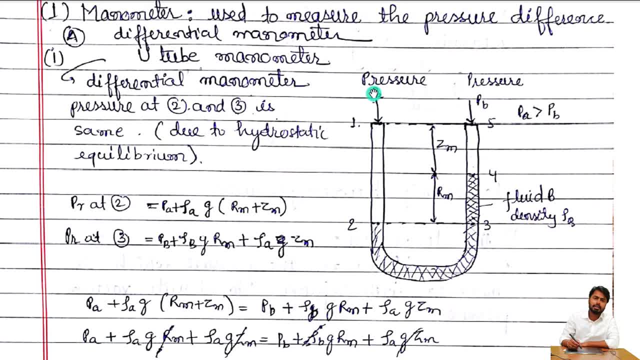 what will be our pressure? if this is atmospheric pressure, then it can be atmospheric pressure, and if it is connected to the system in a pipe system, then the pressure in that pipe will be the pressure right now. suppose our pressure is here, plus because of that, because of the height. 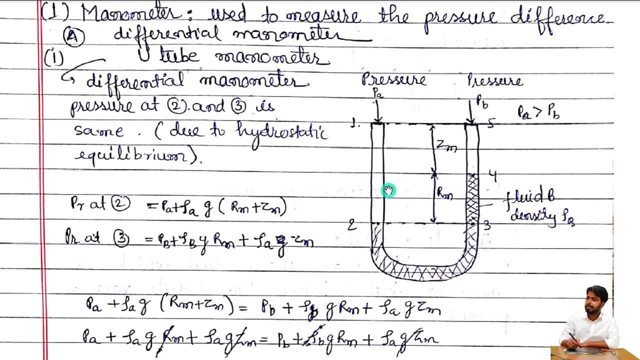 our pressure is coming right because of the height. so what is our height? zm plus rm will be our net height. so rho into g into h. so what is the density of rho a here? rho a into g into h, what is our h? 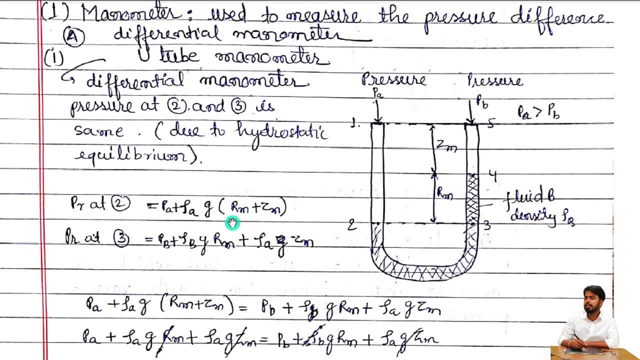 rm plus zm. total height: h. so instead of h we have written rm plus zm, so pressure at point 3. so if you calculate the pressure at point 3, then here is the pb. this will be the pressure plus this height, this much pressure into what will be your. 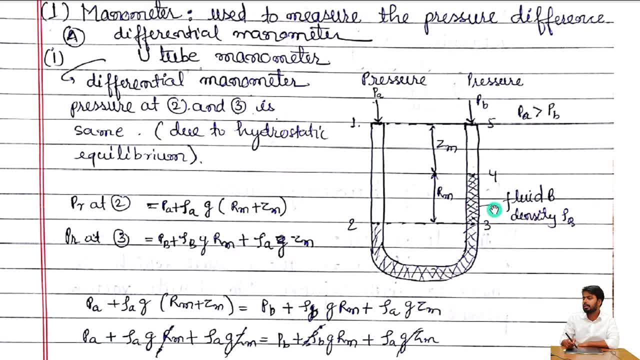 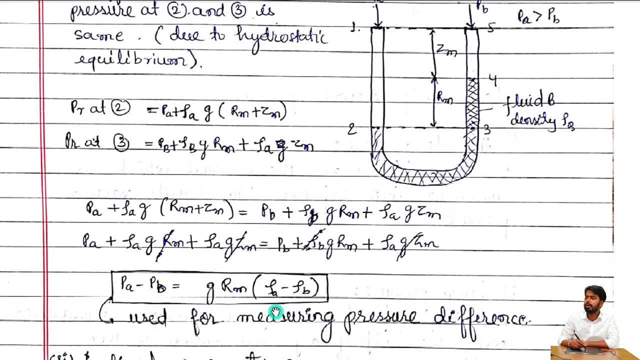 rho a into g into zm. second is, what is the density from here to here? because rho b into g into rm- now we have to do the cross sectional area is same, so we will neglect it directly. so what will you do? equalize these two after equalizing the net value. 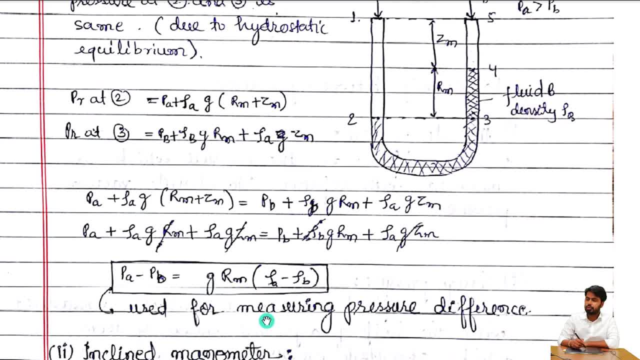 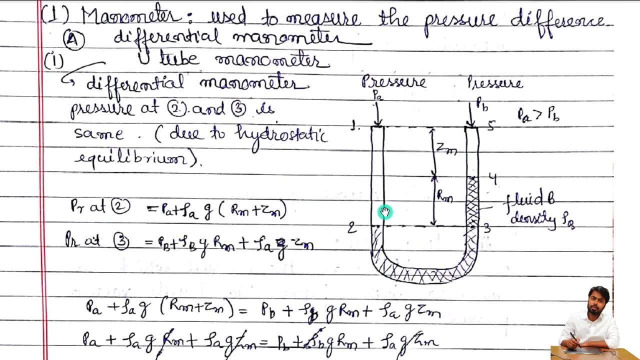 pb minus pb, equal to grm rho a minus rho b. so this is used for measuring pressure difference. so this is the derivation of youtube manometer. many times the problem of base numerical is asked on this. sometimes 2 or 3 fluid will be given inside. 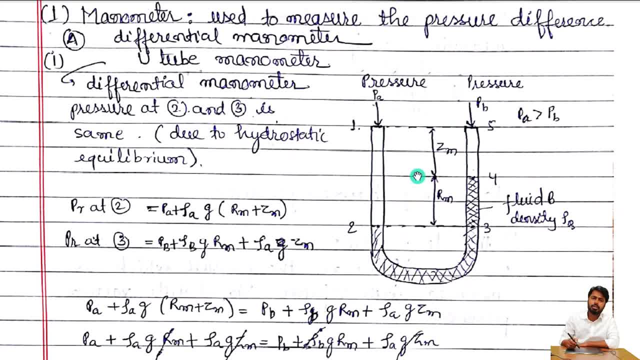 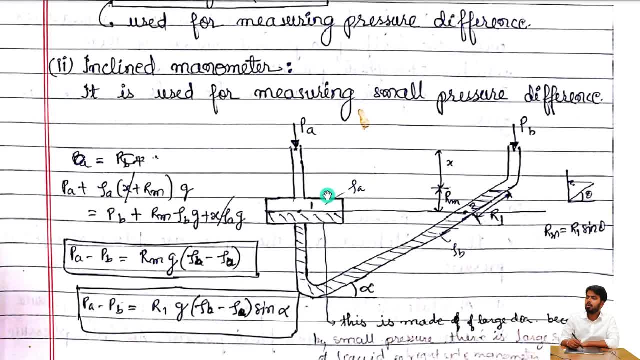 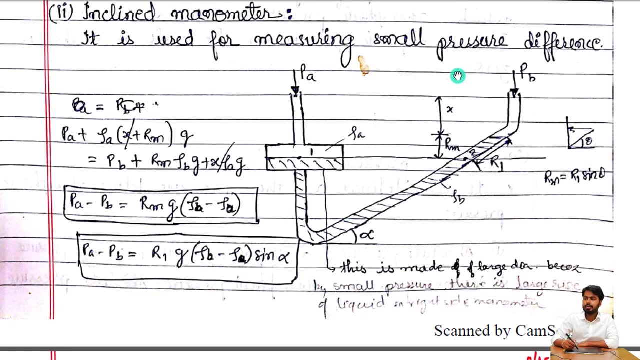 here cross sectional area will be given, more here, less so base numerical problem on all these will be solved. for the better understanding now incline manometer. so incline manometer is used for measuring small pressure difference. now your density variation is very less so in that case. 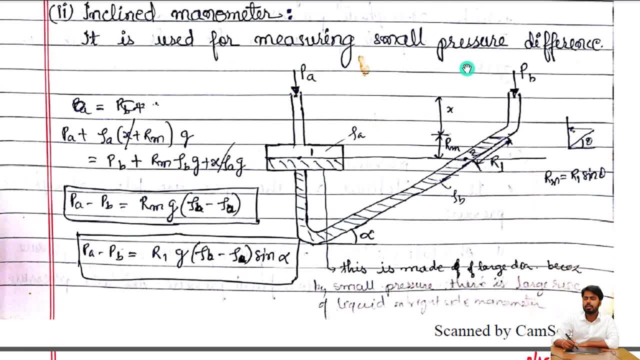 if we want to do small pressure difference, then we use incline manometer and in this the characteristic property of incline manometer is that this section of larger diameter is made. reason is that this is made of larger diameter because by small pressure there is a large rise of liquid. 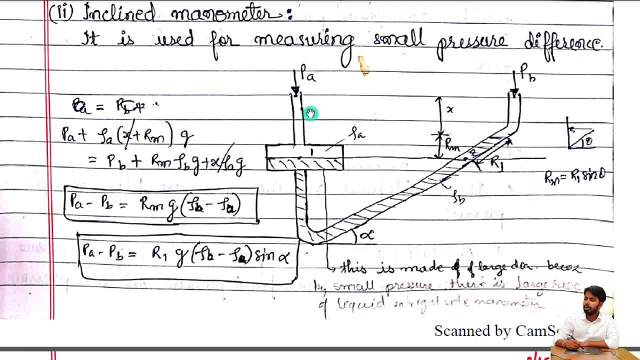 in the right side of manometer means if we do small pressure, then what will happen here? it will go down little bit only, so the volume will be displaced because of this. so we get more height. ok, so our error will be less. ok, then we can calculate the differential pressure. 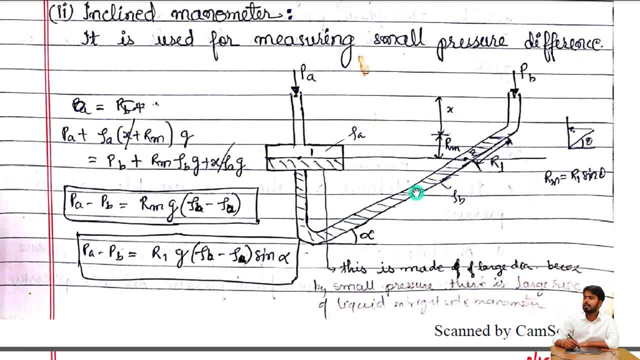 differential pressure. now what we have to do? we have to use same funda. fruit is same. here we have to draw a line under which our density is same. so we draw a line like this. now, at this point, and at this point we have to balance the pressure. 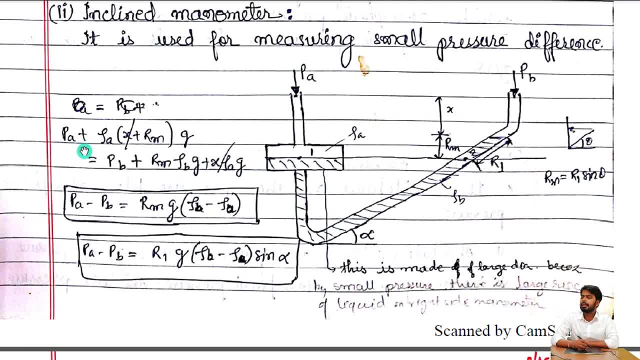 now how much is it? this is P A plus rho A. now how much is the length from here to here? here it is X. so if you take H, then H is equal to X plus R, M, rho G, H, rho A into X plus R M is H into G. 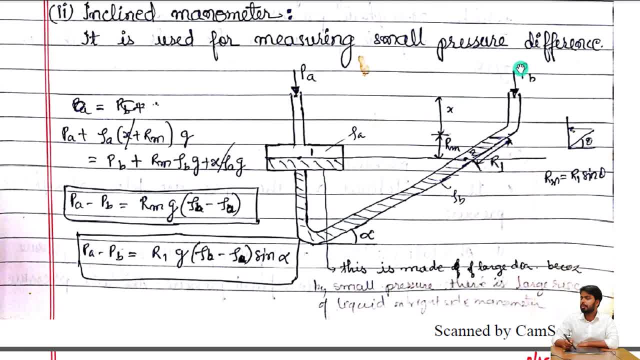 so this side pressure is this: if you take out this side, then what will you take out? X, from here to here from where the meniscus is made. so this first pressure will be P B which will be applied to it, P B plus rho B. its density is rho B into G. 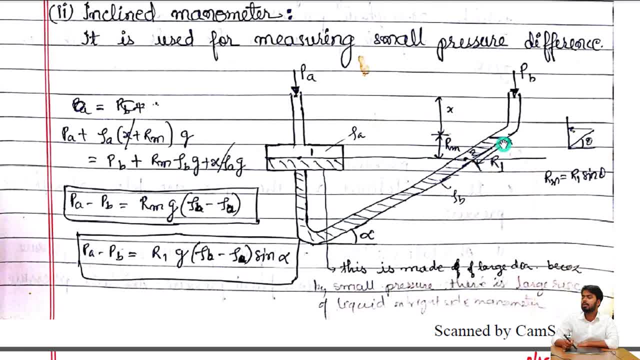 but we will not be given any value like R M. we will see this length in scale. we will see R 1. so what we have to do? first of all we take out this: P A minus P B is equal to R M. G R M into G. rho B minus rho A. 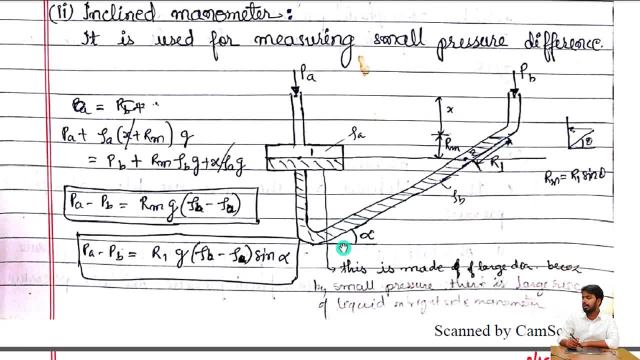 now, what is R M? we will be given R 1. so what is R 1? this angle of incline mandometer, this alpha angle, is always given. so this component will come and the perpendicular component of this Y axis will come: R 1 sin alpha. 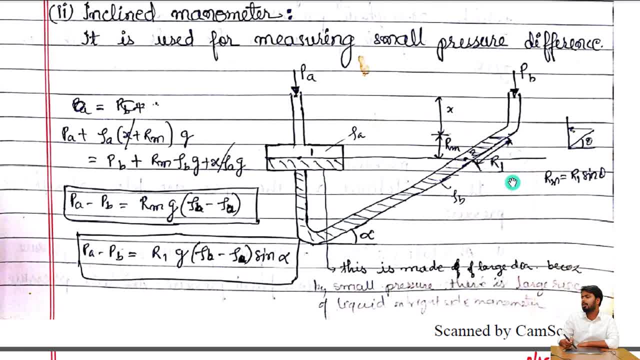 what will come below: R 1 cos alpha, R cos theta and this one. this comes in cos theta and this comes in sin theta. R M is equal to R 1 sin alpha or theta, whatever you keep. if you keep alpha, then you keep alpha. if you keep theta, then you keep theta. 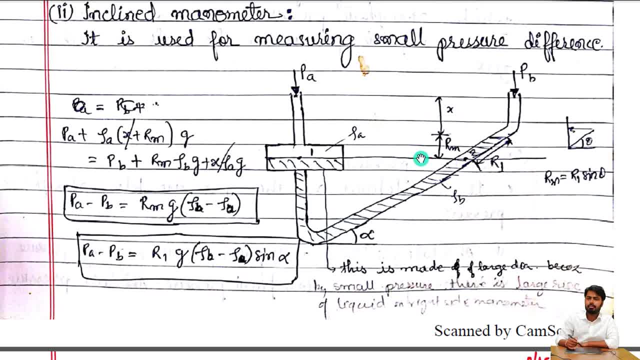 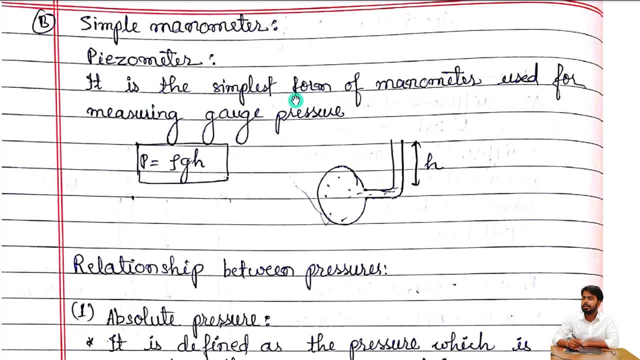 correct? so this is the equation for incline mandometer, correct. now second application is simple mandometer, so this is kind of piezometer. so it is the simplest form of mandometer and used for measuring gage pressure, the gage pressure that is measured. 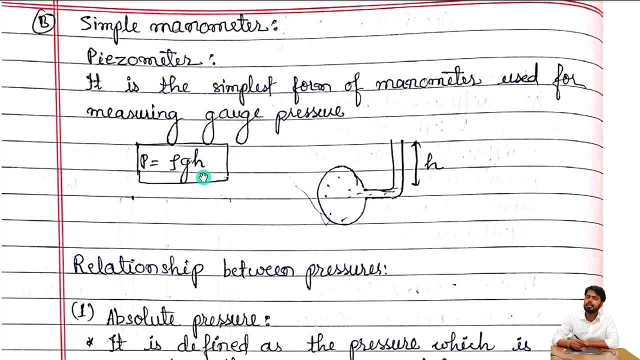 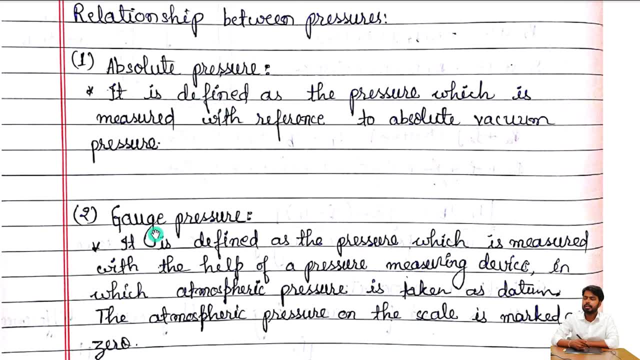 this is the simplest type of mandometer, so pressure is measured like this. into pressure is equal to rho G H. now we will see the relationship between pressure means the relationship between pressure is absolute pressure, gage pressure and the vacuum pressure. so before reading this definition, 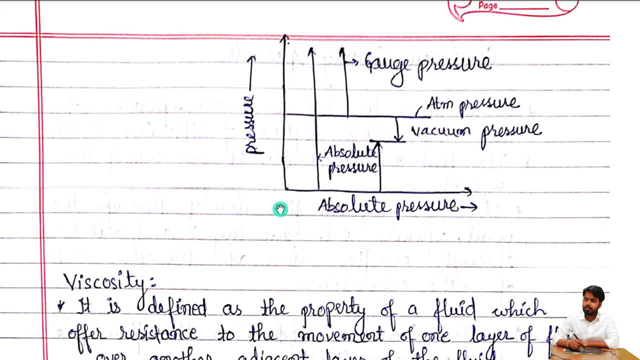 we will see this diagram. so here Y axis is taken as a pressure and on the x axis is taken as absolute pressure means the pressure here is also absolute. this vertical line is absolute pressure. this is also absolute pressure. this is vacuum pressure, this is gage pressure. 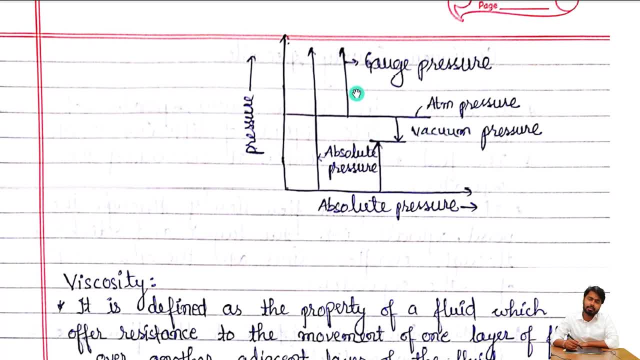 and this datum line is atmospheric pressure, first of all, when your gage pressure- in industry we always measure in pump or vessel gage is written as PG. so what is gage pressure now if you take out absolute pressure? first of all, if it goes above atmospheric pressure? 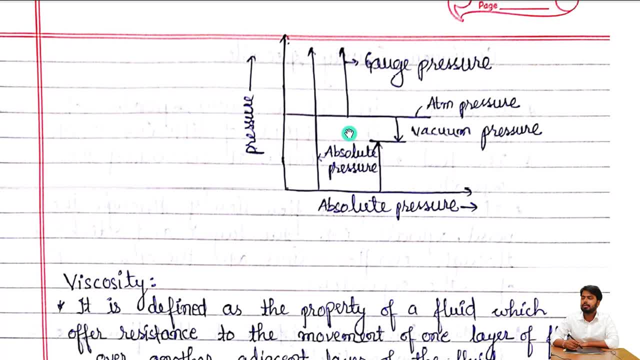 then what will be the absolute pressure? your atmospheric pressure plus gage pressure. atmospheric pressure plus gage pressure, this will be your absolute pressure. second case, when gage pressure will show negative, so the negative value. this is called vacuum pressure in this, so your the vacuum pressure. 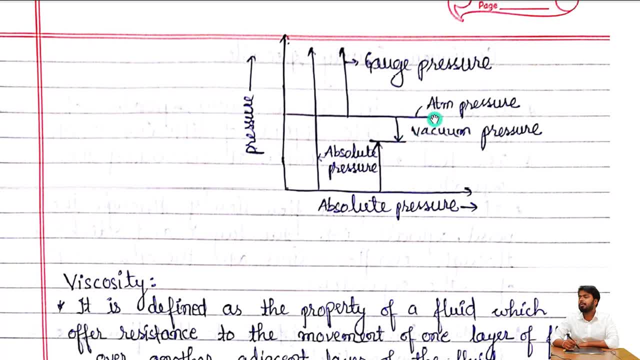 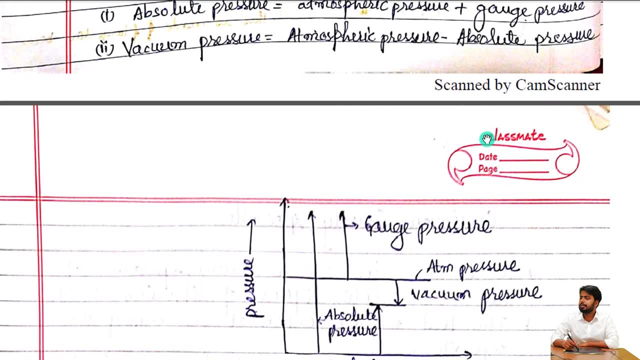 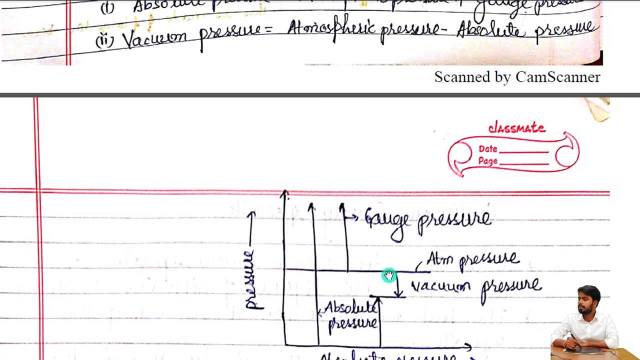 basically, what will be your atmospheric pressure means your absolute pressure, correct? so at this point absolute pressure is equal to atmospheric pressure. right then, what is vacuum pressure? atmospheric pressure from here to here at this point means absolute pressure. so what will be the G a, g, g, g. 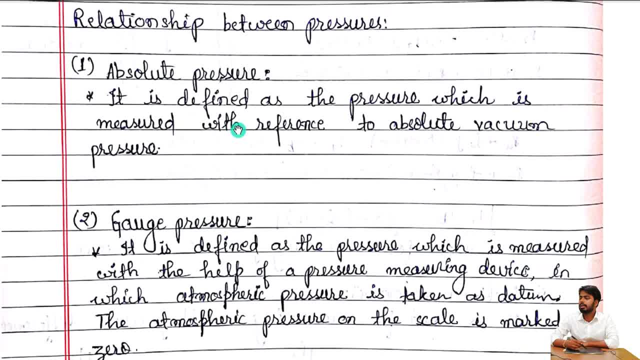 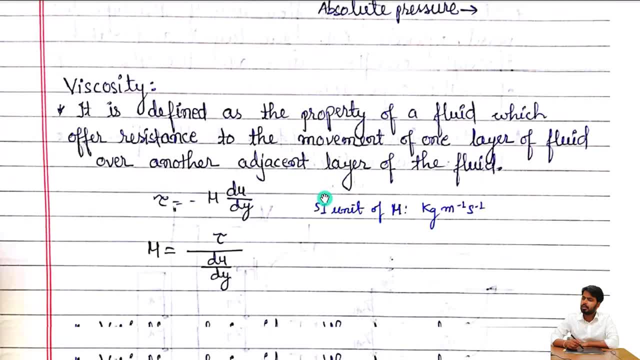 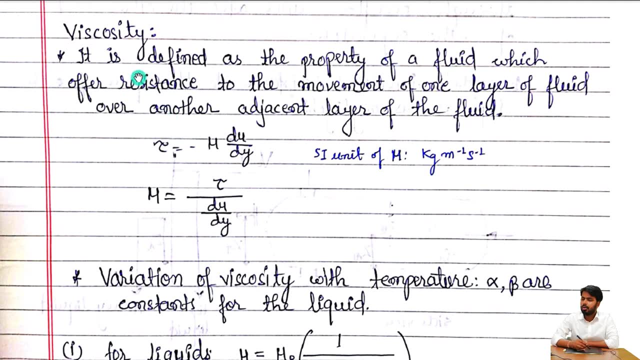 gage pressure. we can read the definition. so this is same as what I said. now coming to the viscosity. so what is viscosity? so it is defined as the property of a fluid which offer resistance to the movement of one layer of fluid over another adjacent layer of. 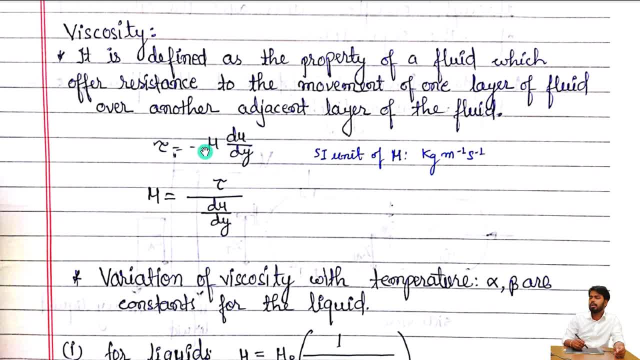 the fluid. so tau is equal to minus mu. dv by dy. what is mu? it is the unit of viscosity. let's show it: tau is shear stress. dv by dy is the gradient of velocity: velocity gradient. so this is the unit of mu. kg per meter per second. so mu is equal to tau dv by dy. 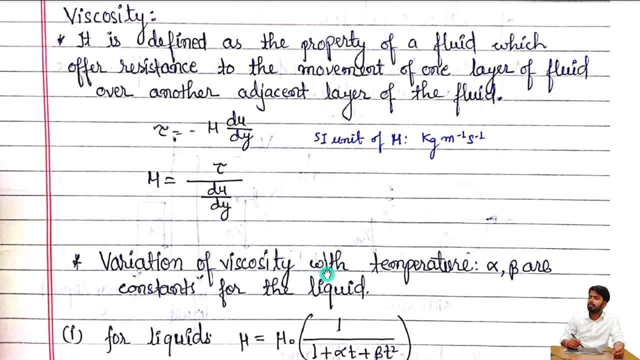 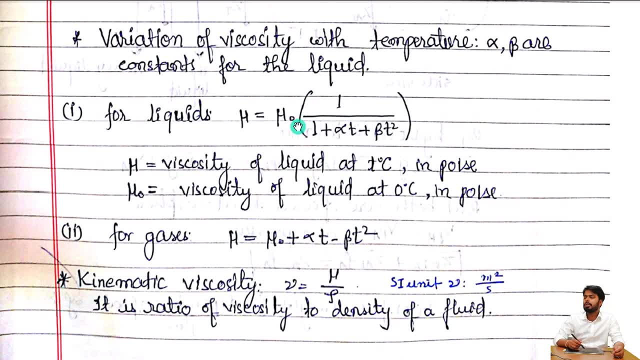 ok, now variation of viscosity. with temperature. alpha and beta are constant for the fluid. ok. so for liquid, the relation given is: mu is equal to mu 0 divided by 1 plus alpha, t plus beta, t square, where alpha, beta is said to be constant. 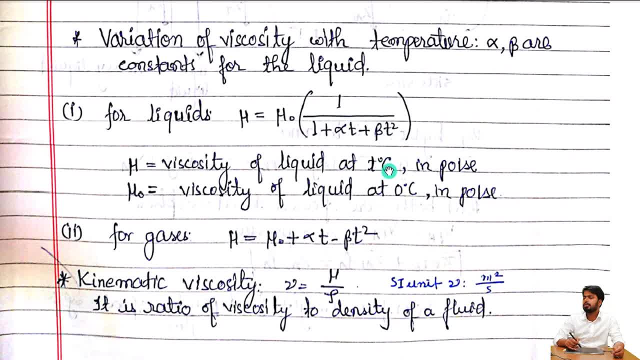 for the liquid. what is the temperature in degree Celsius? viscosity of the fluid at temperature degree Celsius. so the t degree Celsius you have to take in poise, mu 0 is viscosity of the liquid. viscosity of the liquid at 0 degree Celsius. so mu is the temperature that we have to calculate. 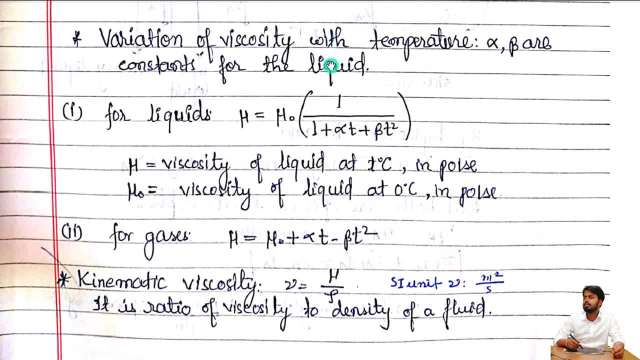 mu 0 is the reference of 0 degree Celsius and you can calculate the value of alpha and beta and you know how much temperature is there. you can calculate the value of temperature for gaseous. this relation follows what is the kinematic viscosity? it is the ratio of viscosity to density of fluid. 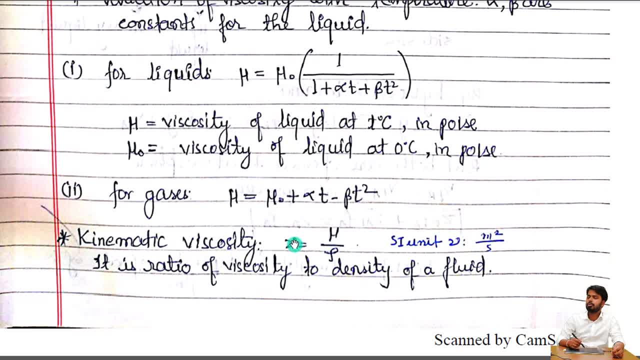 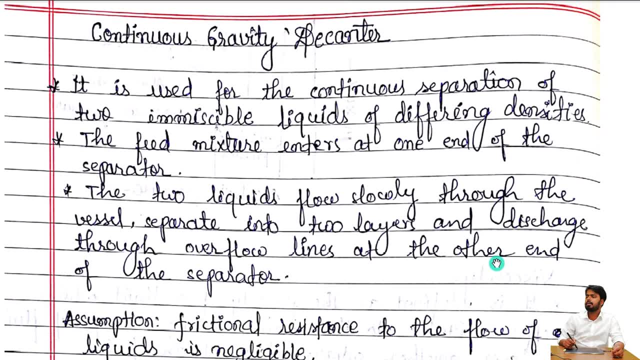 nu is equal to mu by alpha. or another term: mu is equal to nu into alpha. so the unit of nu is equal to meter square by second. now we will see the continuous gravity decanter. so the purpose of decanter is the separation of the liquid based on the density difference. 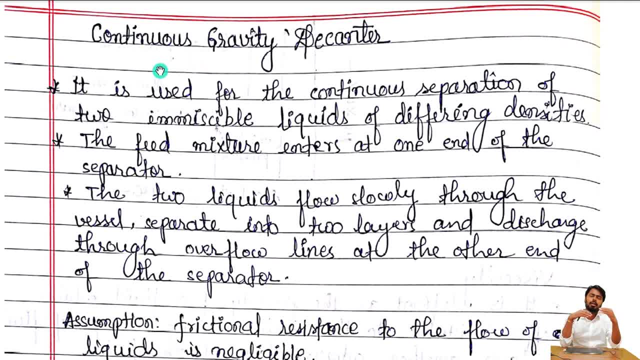 for example, if we take a vessel and put a feed in it, then the feed of different density is entered. so because of the density variation, one layer is deposited on another layer, so an interface layer is formed. so because of the gravity, decanter means the bottom portion of the fluid goes up. 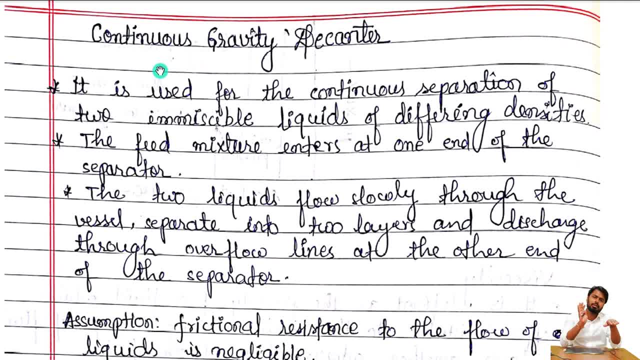 so because of gravity, the higher density fluid will go down, correct? so we have this thing, we call it gravity decanter and if we draw it on continuous basis then it is called continuous gravity decanter. so we can read it here. it is used for continuous separation of two immiscible liquids of different densities. 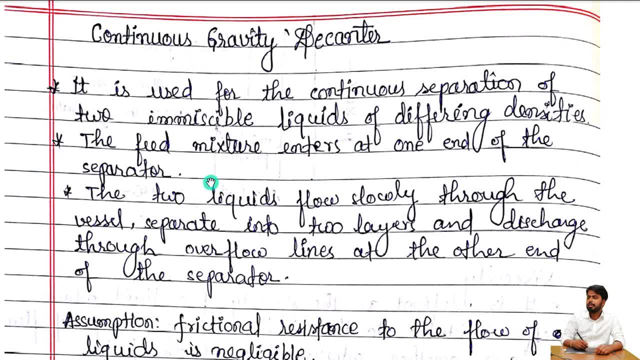 obviously it should not be immiscible. the feed mixture enters at one end of the separator, the two liquids flow slowly through the vessel, separating into two layers, and discharge through the overflow lines at the other end of the separator. so what are the assumptions in this derivation? 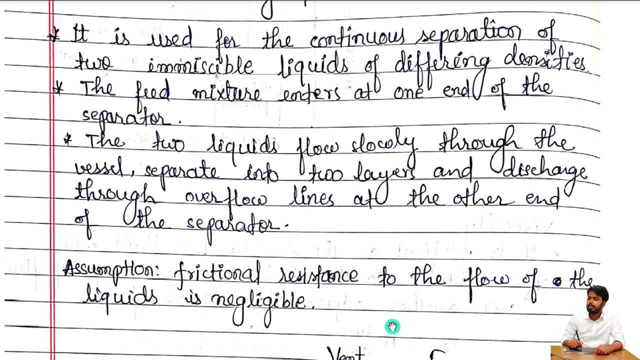 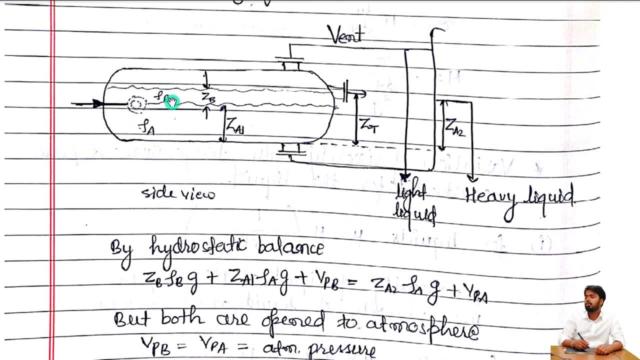 friction. frictional resistance to the flow of the liquid liquid is negligible. so this is the diagram. we are getting the feed. this is the density. the higher density is rho. rho is the load of the light density, z1 is the height of the interface and zb is the thickness of the load of the light density. 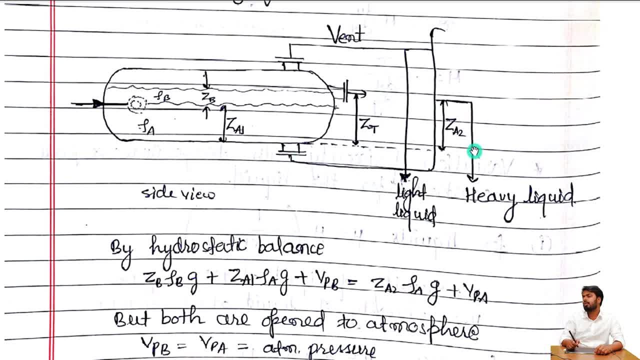 and zt is the total height and z2 is the overflow line where we are withdrawing the heavy liquid. and this is the vent. why do we give vent? generally suppose there is a vapor formation and there are some non condensable gases if there is any temperature in it. 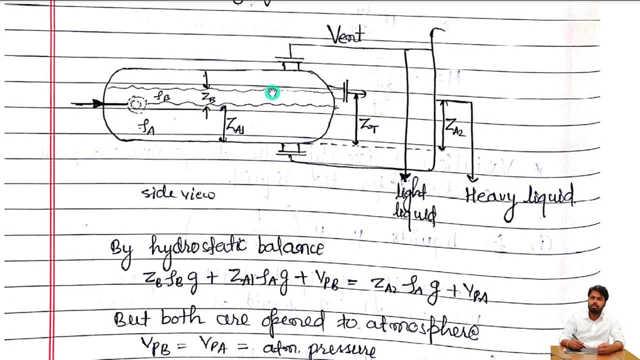 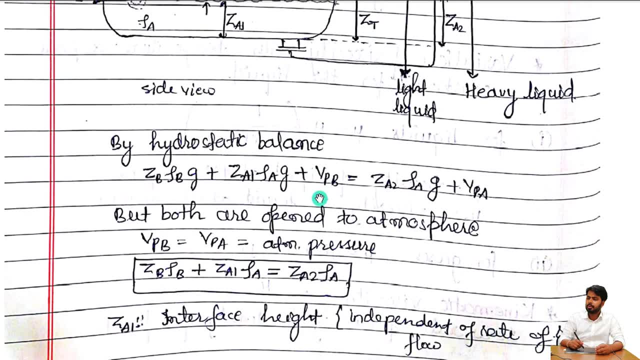 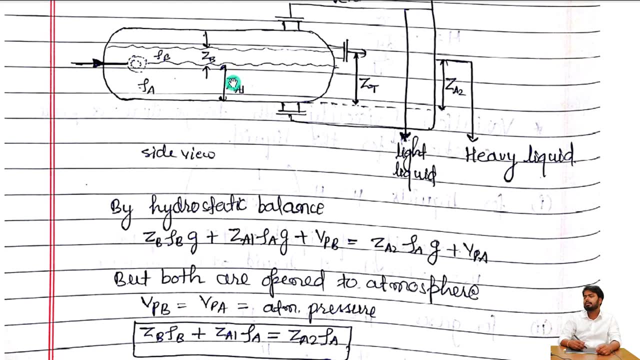 then it starts to operate so that there is no pressure buildup. for that we give venting provision. we gradually remove it according to the vent right. so if we do the hydrostatic balance, what is there? the pressure applied on it. so what was the first? zb into rho, b into g? 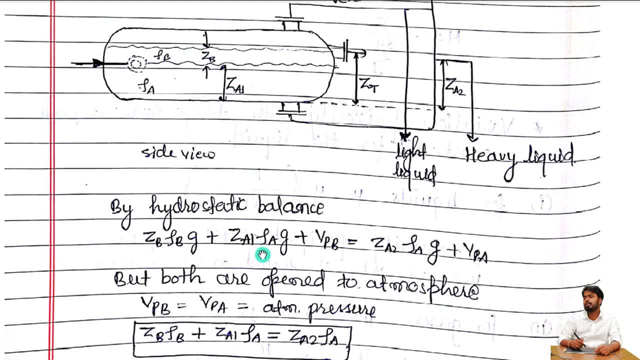 so what is this? zb into rho b, into g plus zan into rho a. its density is done into g plus bpb, so vapor pressure. so if the vapor pressure is exposed to the atmosphere, then what will happen here? bpb means we will count the pressure. now 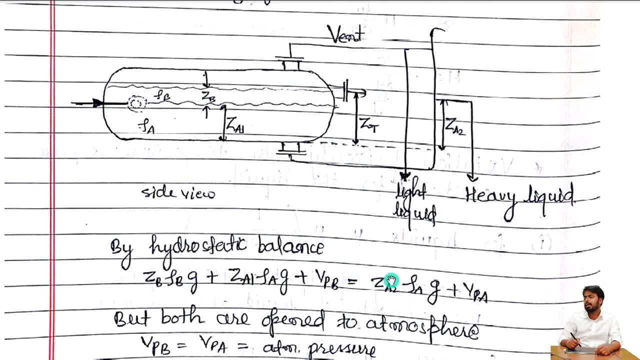 later we will see if there is any vapor pressure flow here now z a2, here z a2 into rho a, because we are taking the density rho a into g plus bpb. now what? but both are open to the atmosphere, then bpb is equal to bp. 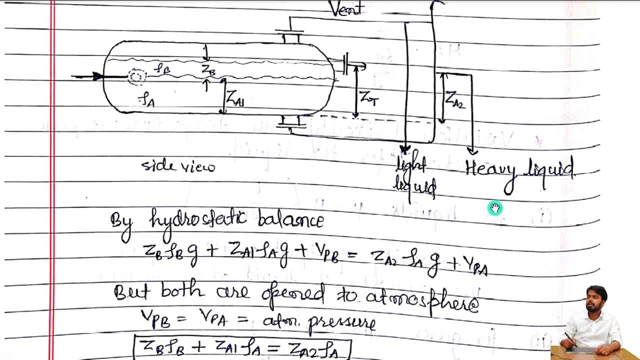 if both are exposed to the atmosphere then both will be the same. closed system is also made and both places are closed system. so suppose if there is more pressure here and there is less bpb, then we will have to take different accountability if we take it in the atmosphere. 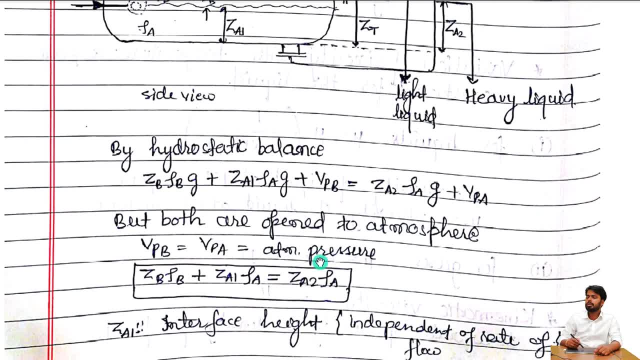 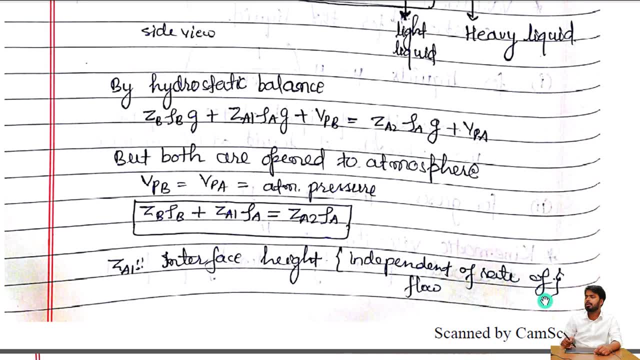 then there is no need to take accountability. both will be the same. so what will happen? zb into rho b plus z a1 into rho a, equal to z a2 into rho a. ok, what is z a1?? it is independent of rate of flow, means it is independent of rate of flow. 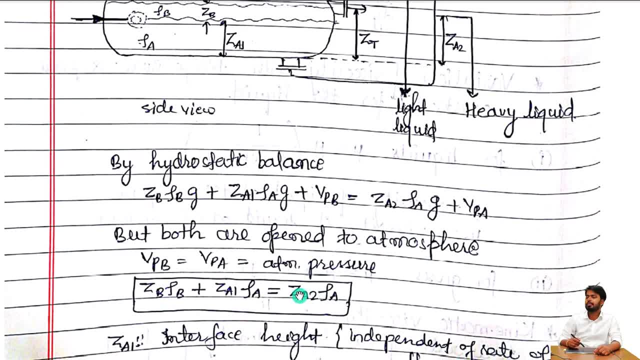 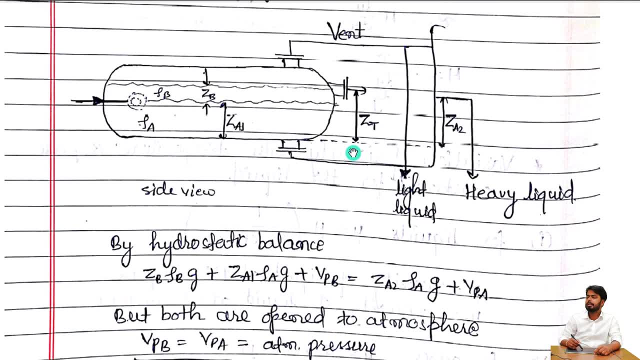 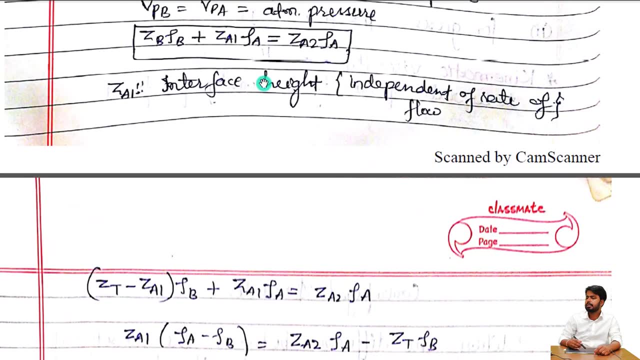 basically, you can see which parameters are dependent on it now. now, what is zb zt minus zan? what is zt? it is totalized. so what is zb zt minus zan correct? plus zan into what is in this zan into rho a. 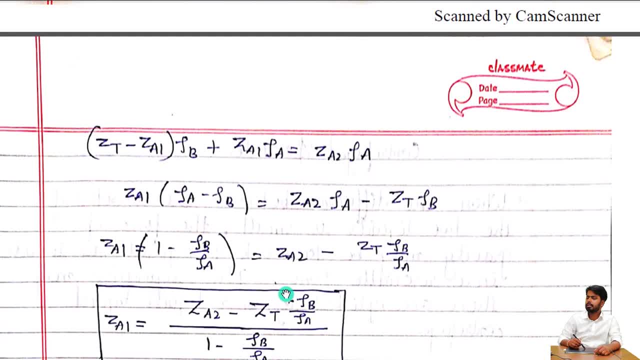 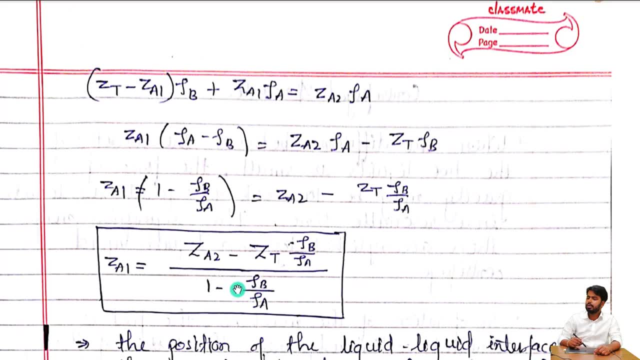 za2 into rho a. now, if we will calculate the value of zan, what will be your value? za2 minus zt into rho b by rho a, divided by 1 minus rho b by rho a. so this is the relation of interface height. what is the relation of interface height? 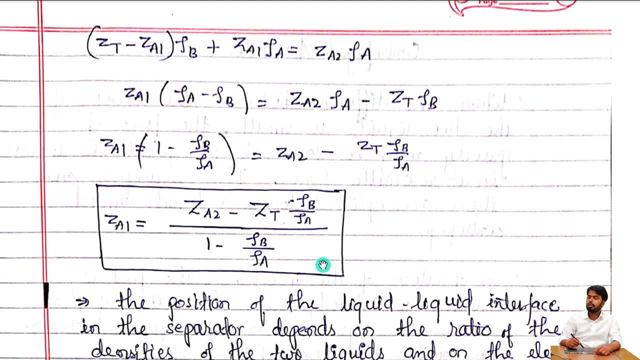 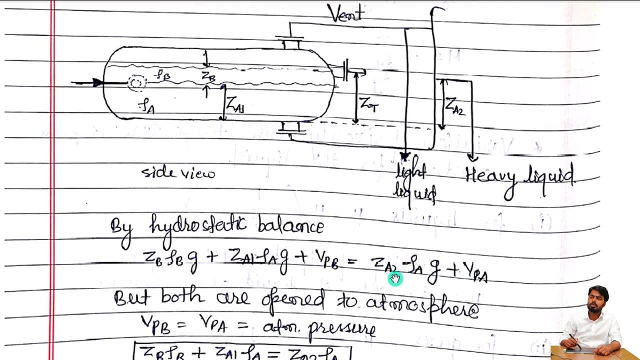 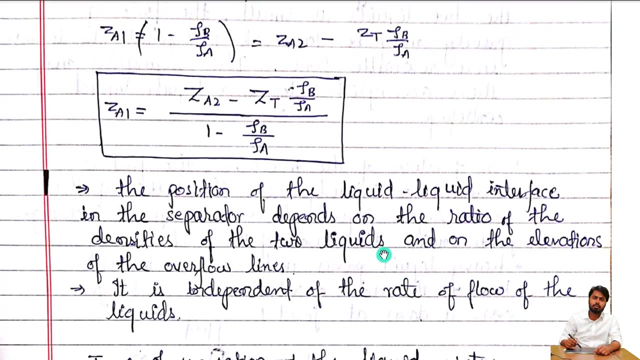 this is the relation correct. on this base, in 2016, there was a numerical means. your configuration was not made like this, but overall the theme was based on this. now this is the question of removing your interface height. in the case of continuous, what is your continuous gravity decanter? 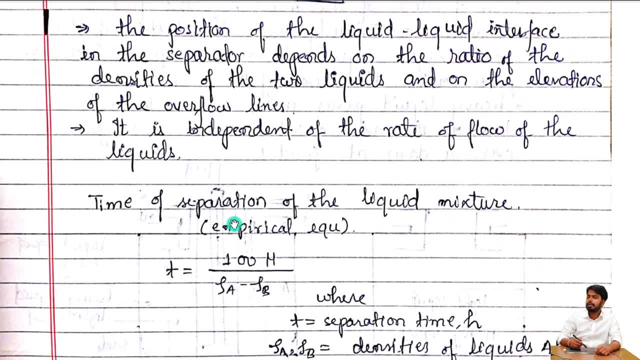 now we will see the time of separation of the liquid mixture. so t is equal to. empirical equation means there is no derivation design by practical. so t is equal to 100 mu divided by rho a minus rho b. what is the separation time here? it will come out in hours. 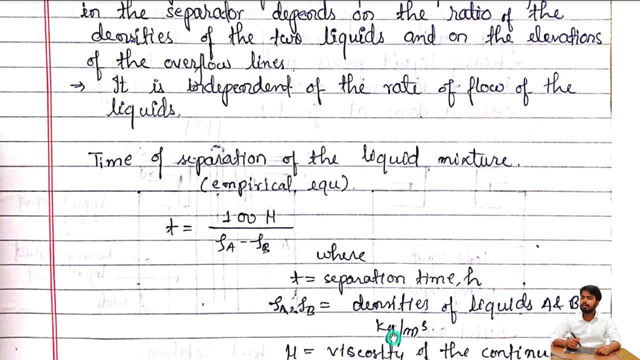 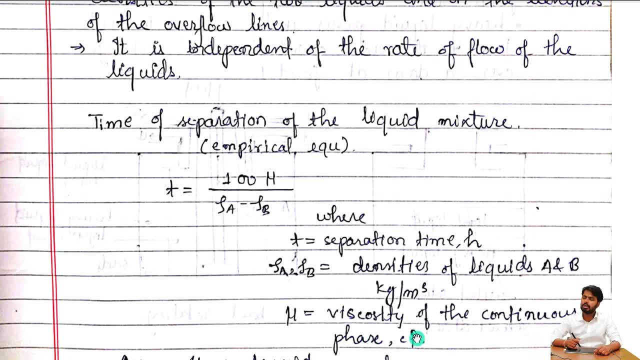 what is the density of rho a and rho b, of a and b, it should be 1 kg per meter cube. what is mu? viscosity of the continuous phase. what is the viscosity of the continuous phase? we have to take that in CP, in centipoise. 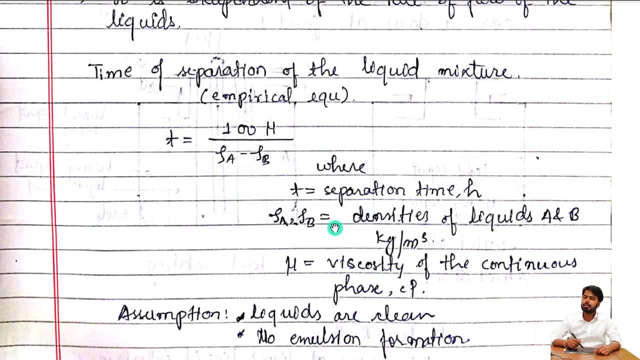 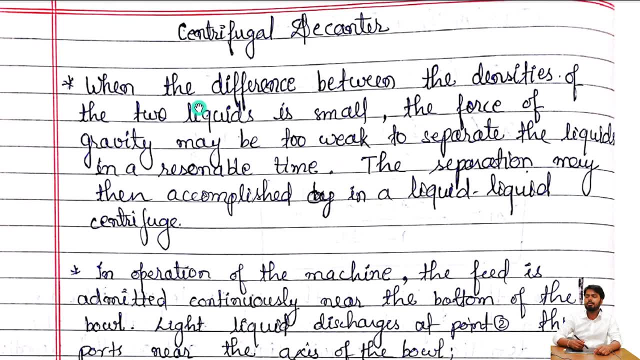 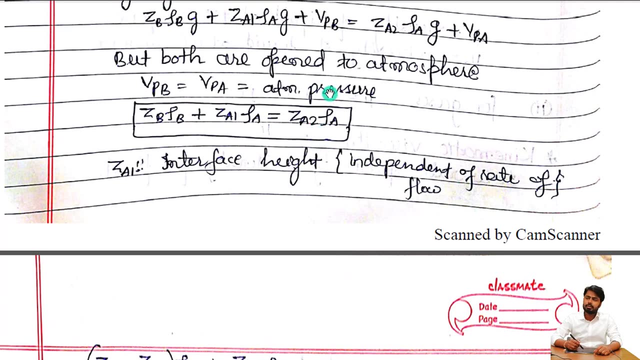 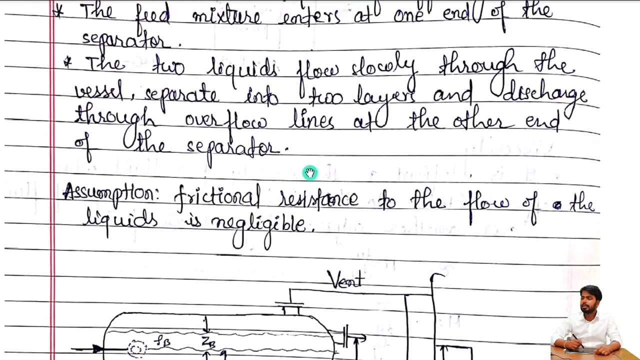 what are the assumptions? liquids are clean and no emulsion formation. these are its assumptions, correct. now we will see the centrifugal decanter. now we have seen gravitational decanter. first we have seen hydrostatic equilibrium, then we have seen centrifugal equilibrium right now. what we have seen here? 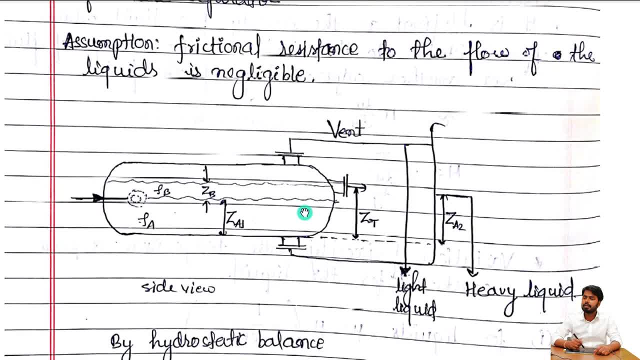 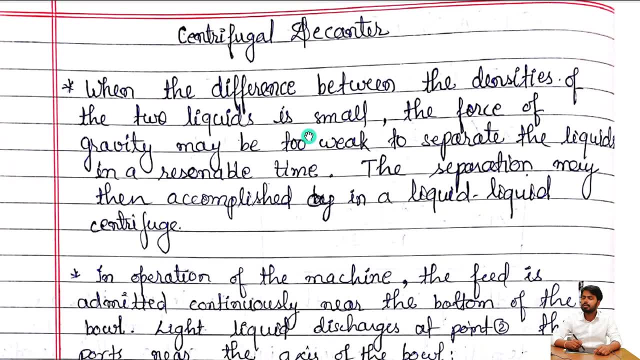 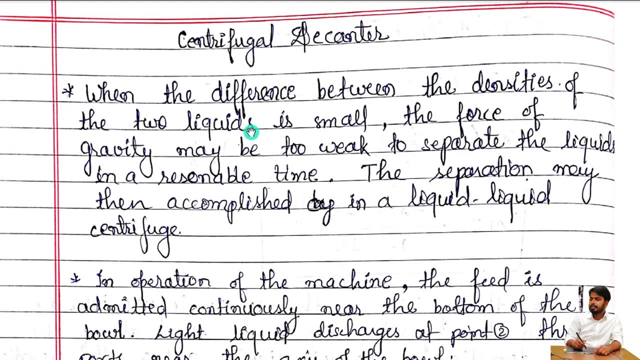 on its application: continuous gravity decanter, so hydrostatic equilibrium. based on it, we will see the application which we call centrifugal decanter. so you can read it here. one, the difference between the densities of the two liquids is small. the force of gravity may be too weak. 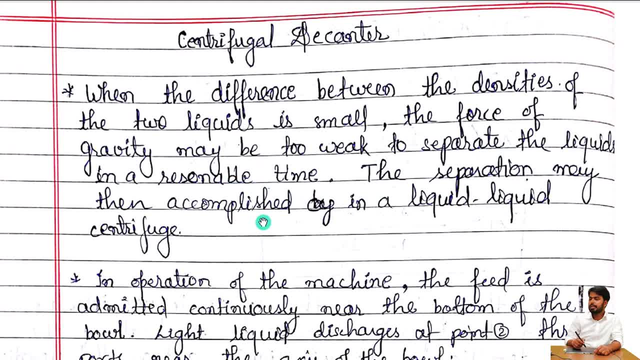 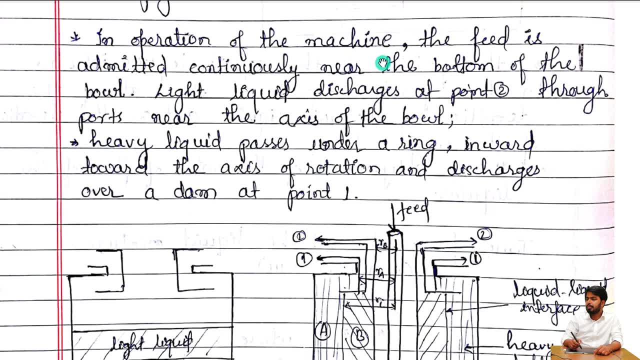 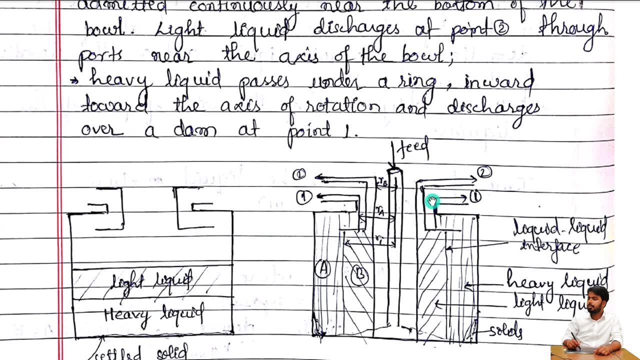 to separate the liquids in a reasonable time. the separation may then accomplish in a liquid-liquid centrifuge correct. so in operation of the machine the feed is emitted continuously near the bottom of the bowl. light liquid discharge at point 2 means our feed will always come to the bottom. 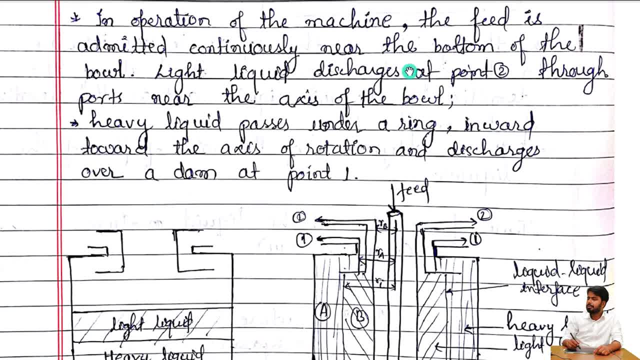 the light liquid will discharge at the point 2, so light liquid will be discharged here and heavy liquid will be discharged from here. ok, heavy liquid passes under a ring inward towards the axis of rotation and discharge over a dam at point 2, so it will be discharged at point 1. 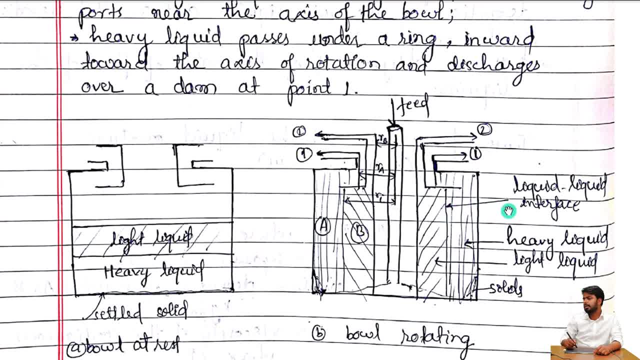 correct. so this point is being made here. let's see what is this liquid-liquid interface, this portion here, because your heavy liquid has been made. this is your light liquid. here some solids are deposited so it can be made a little on the corner and the feed is coming here. 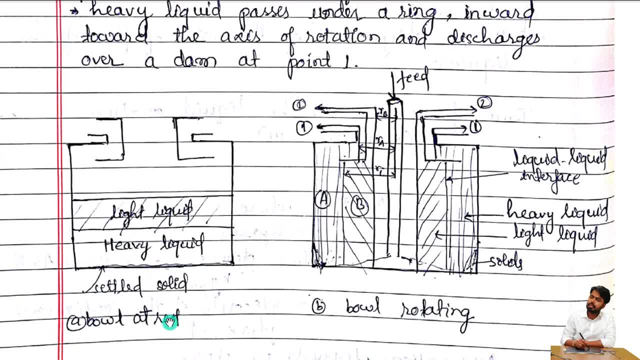 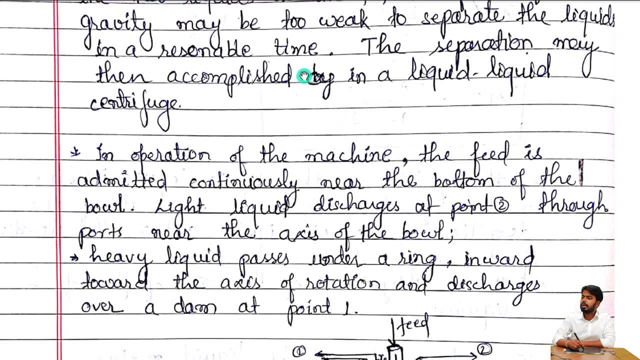 right now. what is this condition? when the bowl is at rest means the bowl is at rest, there is no motion, so the heavy liquid will go down and the light liquid will stay above. correct? what is the density variation in this? it is said that it is very small. 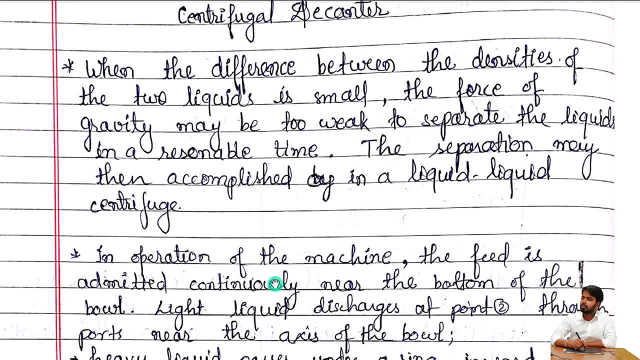 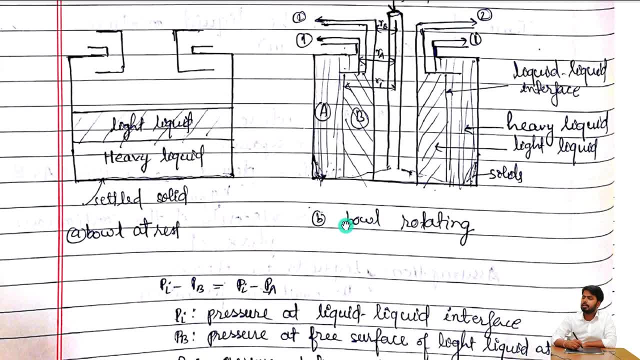 so we cannot separate it from the gravitational force. so we will use the centrifuge. correct now, we will use the centrifuge, so its arrangement will be like this. so the PI minus PA that you have to make, PI minus PB, PI is your interface pressure. ok, because 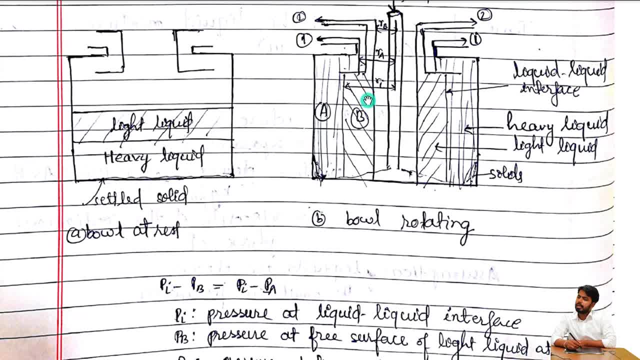 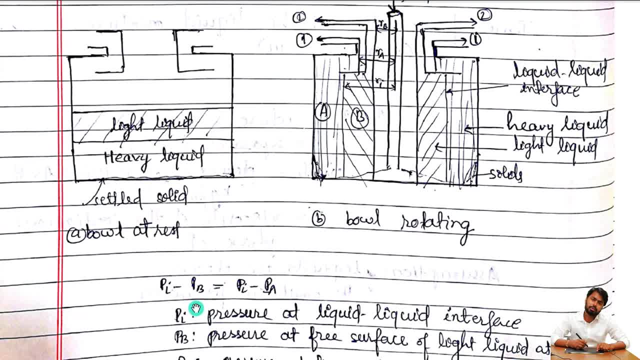 should be constant, so the delta P should also be constant. the velocity should be constant. then PI minus PB, PI is done minus PB at pressure B is equal to PI minus PA. PI minus PA. now what is PI? what is the pressure at the liquid, liquid interface? what is PB? 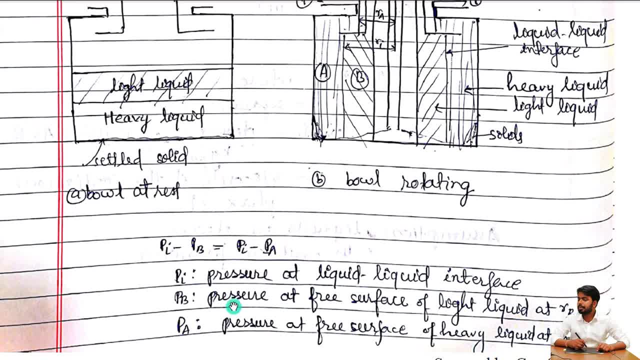 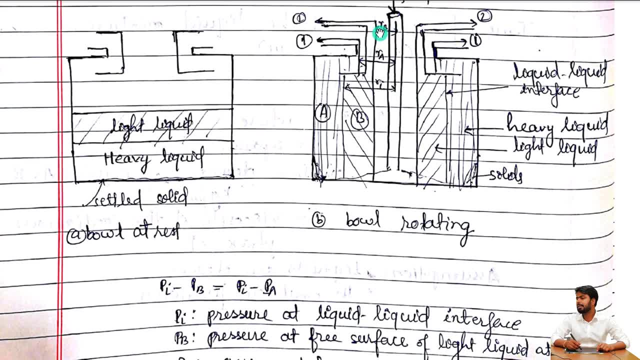 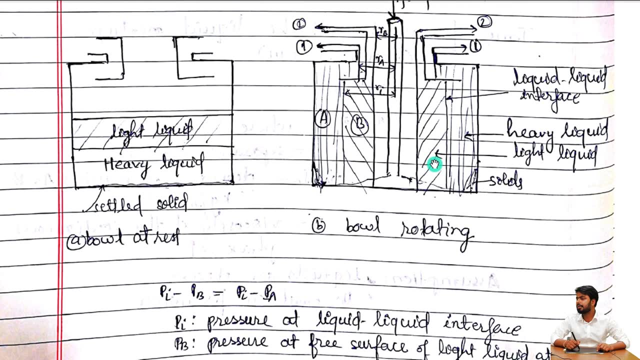 what is the pressure at the liquid liquid interface? what is PB pressure at the free surface of light liquid RB? light liquid RB, that is your RB at the free surface? what isuuuu correct and What is PA Pressure at the free surface of heavy liquid Access? pressure at the free surface. 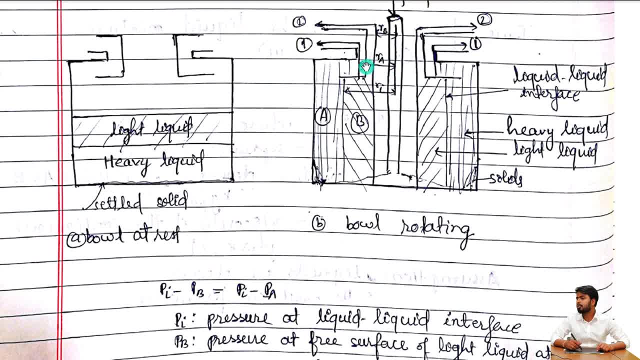 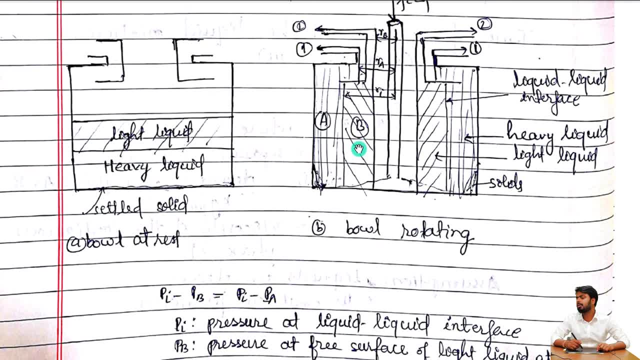 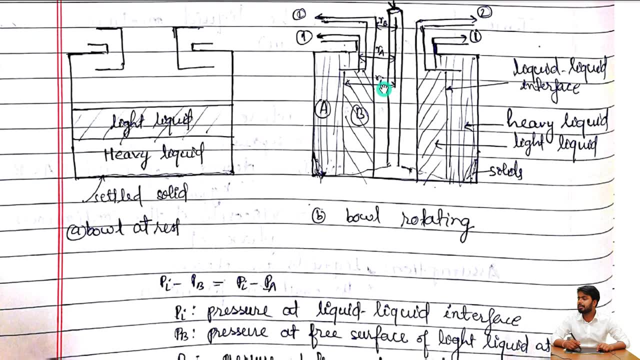 of heavy liquid Is coming coming, So both the free surfaces are exposed to the atmosphere. ораP, The free surface, means Bell number. bar delta P will come same, whether your non-l 이해 why, because it is free surface exposed to atmosphere, is done in free surface, correct. 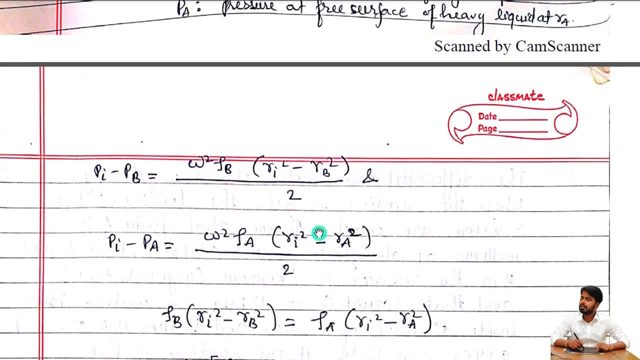 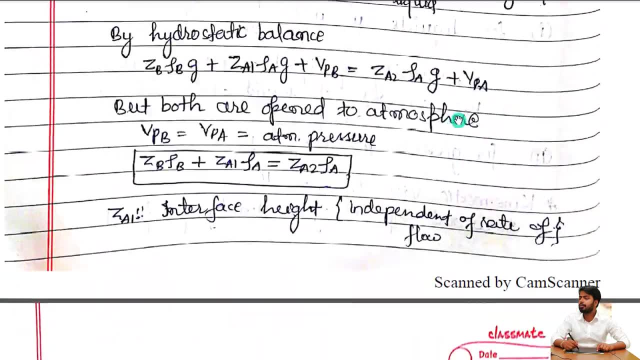 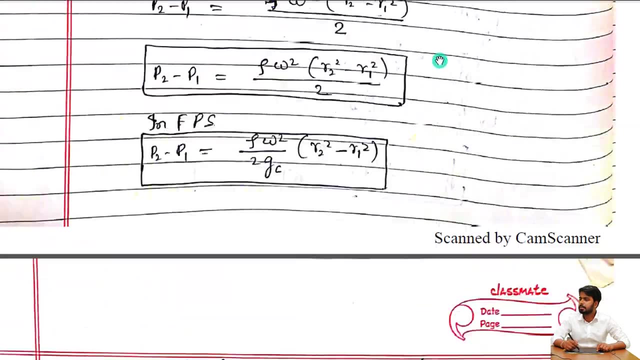 so its delta p will also do pi minus pb. so this relation will come and pi minus pa will do so. this relation will come from where it is coming, from the centrifugal force. in that case the balance we did where it is gone. this is the relation we did in the hydrostatic 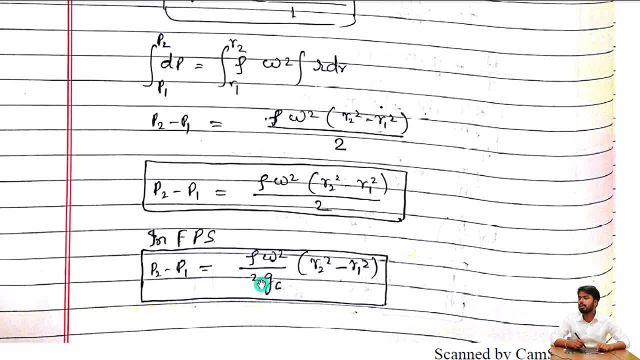 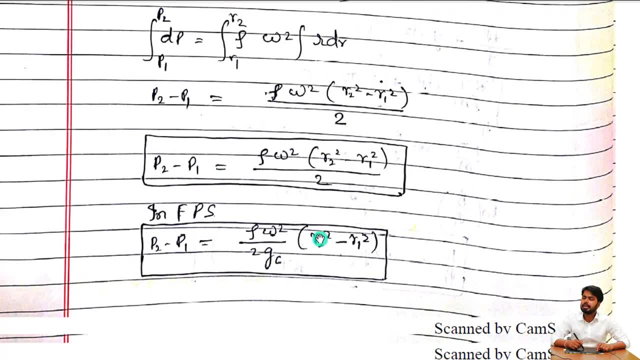 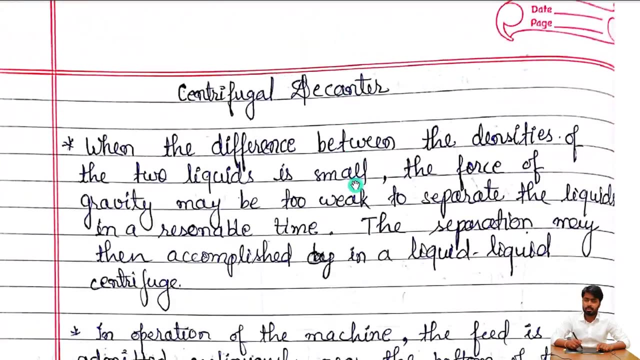 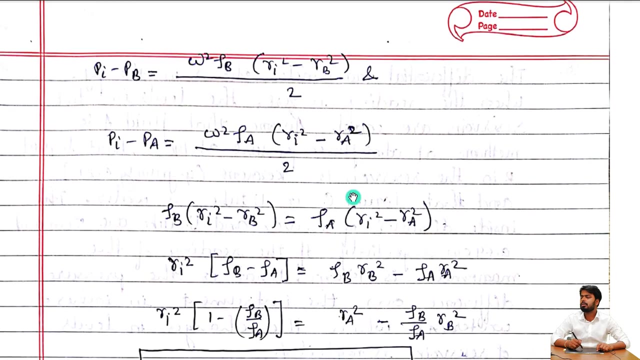 equilibrium centrifugal field. we have to use this relation: pi minus pb, pi minus pa. now what we have to keep. instead of pi minus p1, we have to keep pi minus pa and once b correct. after keeping both, what you will do is equate it after equating, when you solve it, the interface. 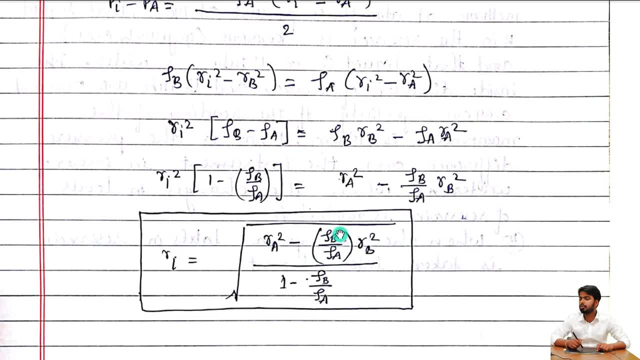 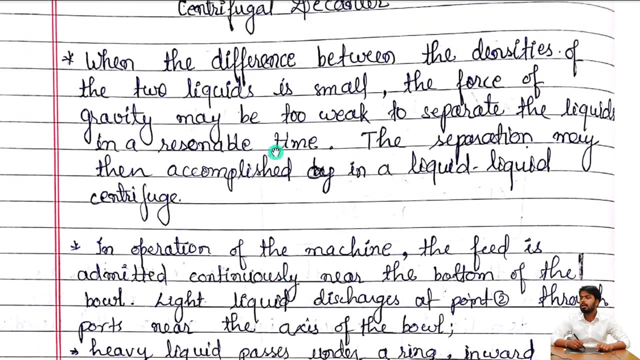 radius of ri is equal to, under root ri square minus rho b, divided by rho a, into rb square whole divided by 1 minus rho b by rho a. ok, when you will do under root of the value of ri, then you will get the value of ri correct. so this is the centrifugal decanter principle. 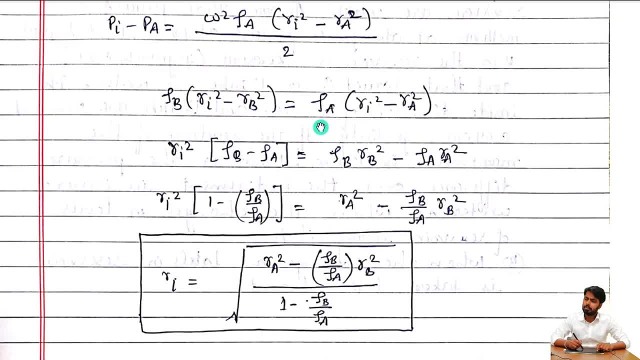 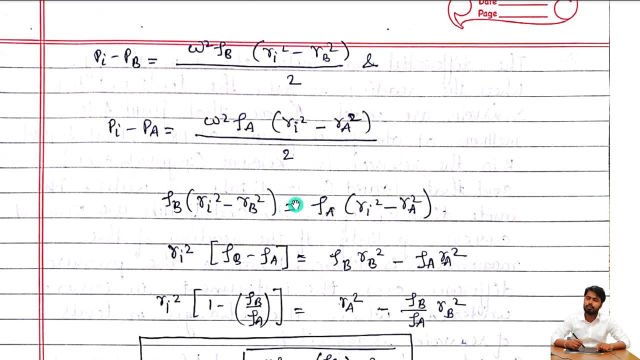 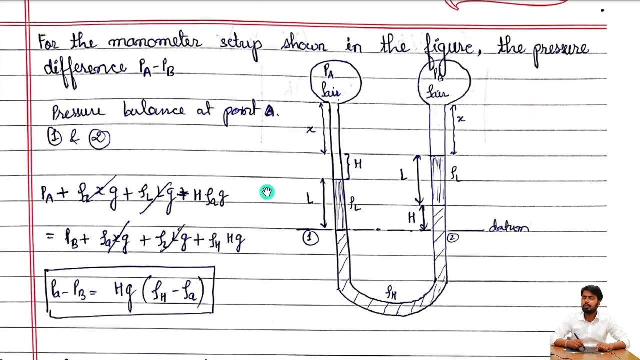 whoever will follow this relation. ok, this pressure difference will be in the hydrostatic equilibrium in the centrifugal field and according to that we can get the radius of the interface by this principle correct. now we will see the application of hydrostatic equilibrium between two, so you. 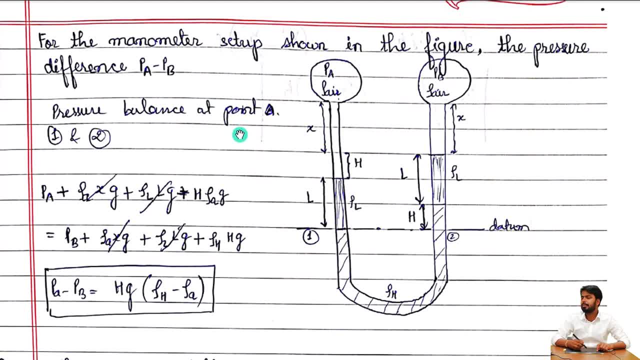 can see it here further better. setup shown in the figure: the pressure difference pi minus pb. so i will get the pressure by pi minus pb. what is there now? there is not exposure to atmosphere correct in such x and y operation. with this there is a に for the pressure bell. 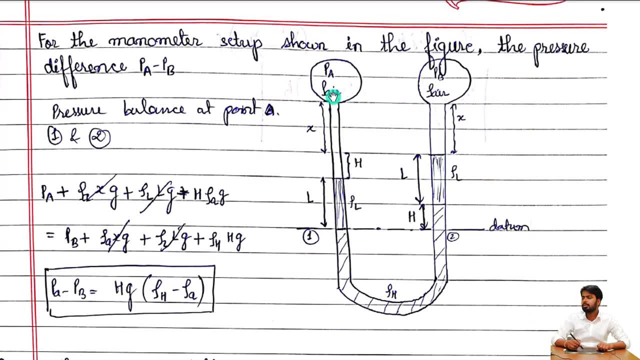 and cry for that very simple note and plus nous not added at that time, given the mass. So what we have to do here? first of all, I said that at such a point where your below will not have its density variation, then a data line will be given immediately. then 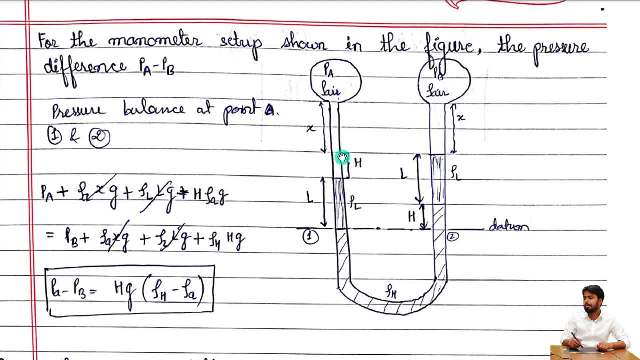 write the pressure on it, write it as a solid. it became PA. what is the distance? we have assumed X, X has become from here to here? this distance is H and this is L. total height is H Rhogh. then, in terms of X plus H plus L, we have to write it as mundo in terms. 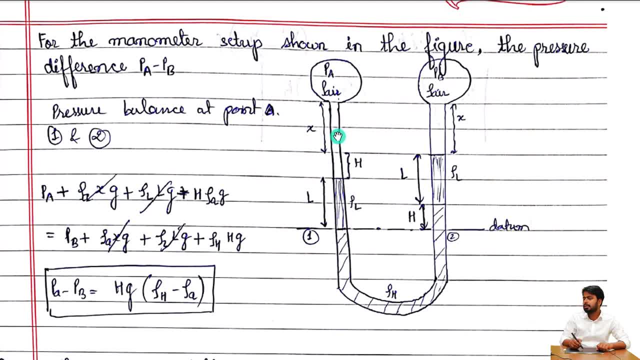 then, in terms of Rho A into X, what is the density? Rho A is Ntux X into G plus H is the same, H into Rho A, into G. now, what is the density here? it is Rho L, so the density of RHO is: 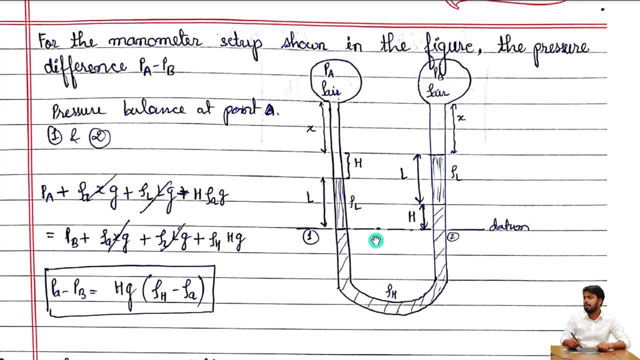 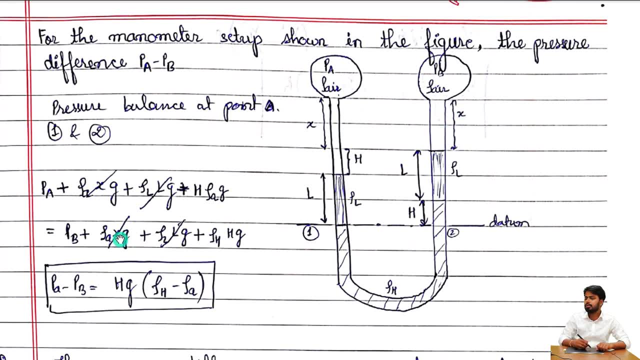 L into G. this is the information you have at this point and the pressure which will come at the point 2 will come. P will also come, X into Rho, X into needing will come into G and X and it will come to the point 4 and in intro, G. this will come to the middle. 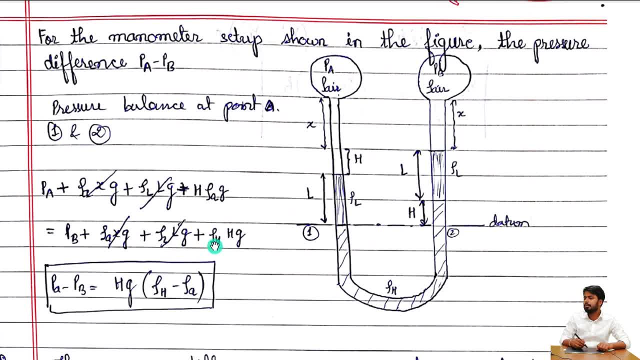 the pressure on point 2 will happen. what will happen? Excel channel X into Rho A into X into Rho A. you will get the K 0, E because now the pressure on your manual has come into your manual. this will be: Rho L into L, into again G will come plus Rho H into H into G will come correct. 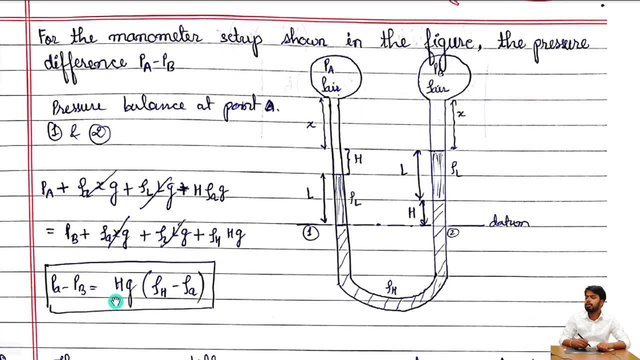 if you equate these two, then your P A minus P B will be equal to G H Rho H minus Rho A. so this will be your actual relation. so what does it mean if the liquid of the same density comes in between these two means this extra part will be L Rho L. 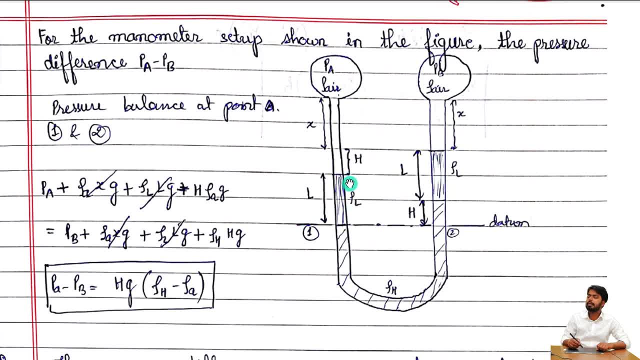 and here L Rho L, we can directly eliminate this, so our first relation can be directly used. so this is basically based on the concept of how much your brain works. then, accordingly, you can solve the question. it is basically based on the knowledge of your brain and your practice. 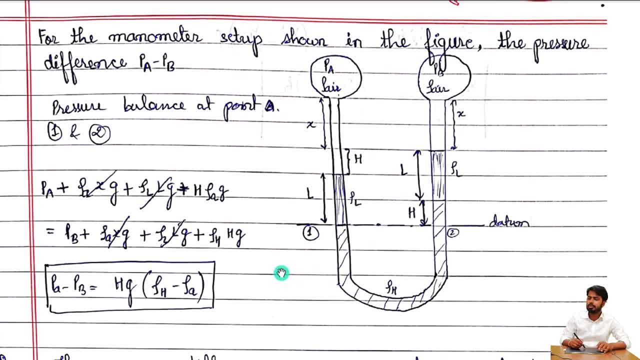 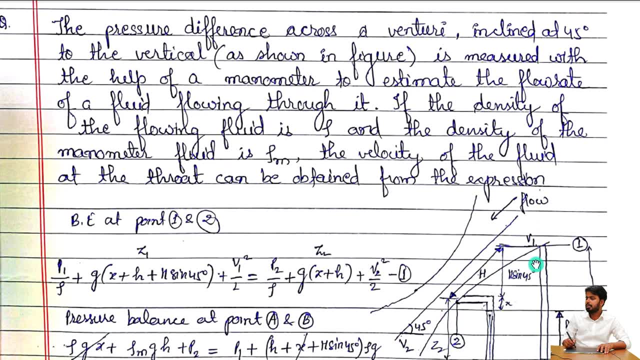 number of question. you solve more, you have to solve more, you don't have any other option. ok, now the second question: the present difference across a venturi. you can see this venturi and this is throat, and this is expandable. The pressure difference across the venturi is inclined at 45 degree to the vertical is 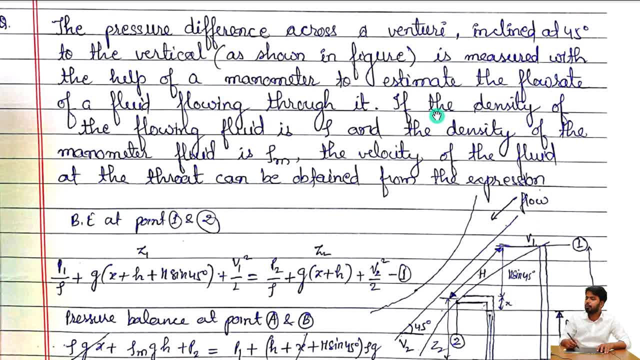 measured with the help of a manometer to estimate the flow rate of a fluid flowing through it. If the density of the flowing fluid is rho and the density of the manometer fluid is rho m, the velocity of the fluid at the throat can be obtained from the expression. 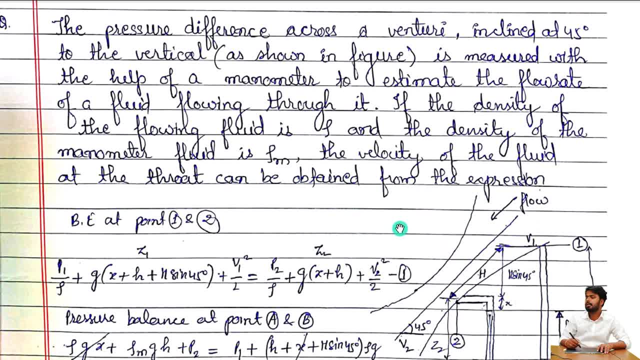 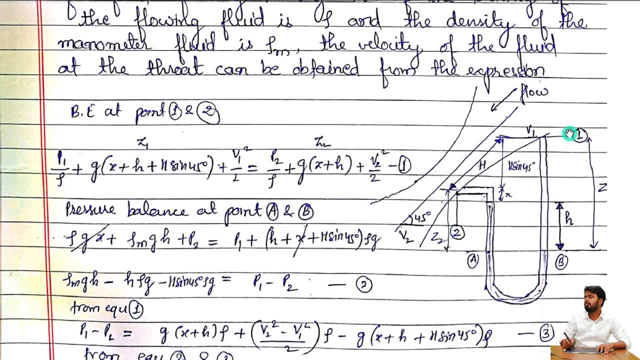 So basically, we have to find the velocity at the throat. so you have to find two simple relations here. First of all, use the Bernoulli equation on point 1 and point 2, so point 1 is ours, point 2 is ours. you have to use the Bernoulli equation on these two. so what was the Bernoulli? 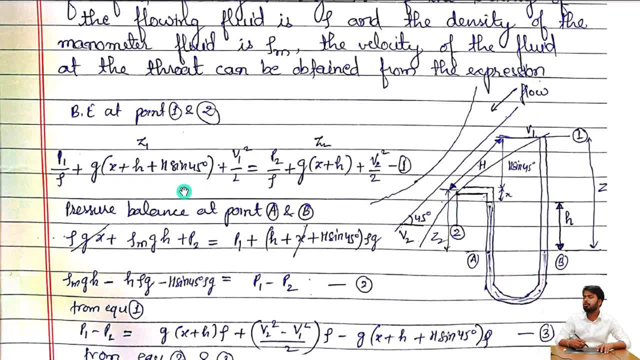 equation p1 by rho, where p1 by rho plus gz. so what will happen to you? which is your reference point? suppose we took the reference point from where. this is our reference point, correct? so this is point number 1, we have taken this one. now what to do with this? 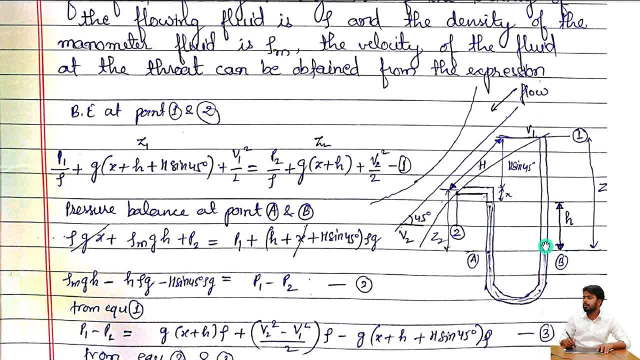 z1, so what is this in z1, I have taken one h of yours. second, I have taken the portion of x. third, if the value of h is 45 degrees, then what will happen? h cos alpha is h sin. 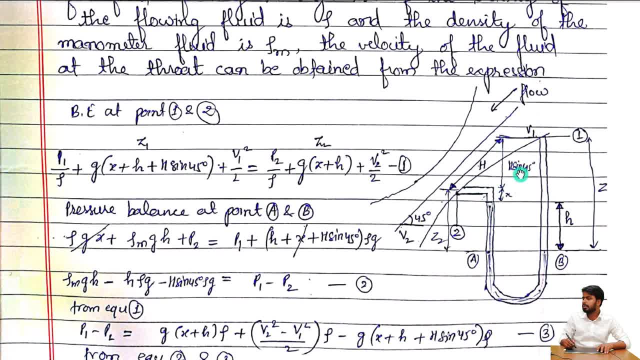 alpha. so this portion will be given as h sin 45 degrees will come. so h sin 45 degrees plus x plus 45 degrees will come. So this is the reference point. So this is the reference point. So this is our reference point. z will be given from here. so we have taken it. and what is? 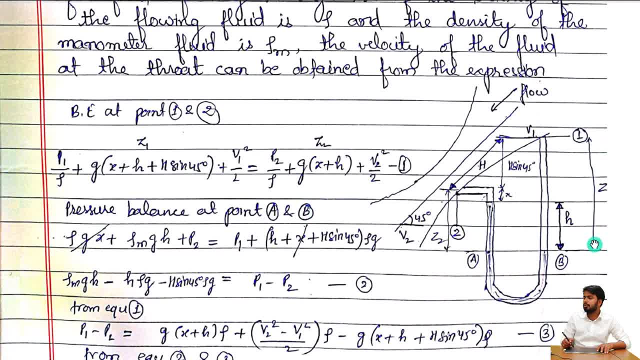 the value of h, the value of h will come. total. z means z1 means from here we have taken 1, z means it will be z1, so it will be v1 square. so the velocity at this point is v1, so it. 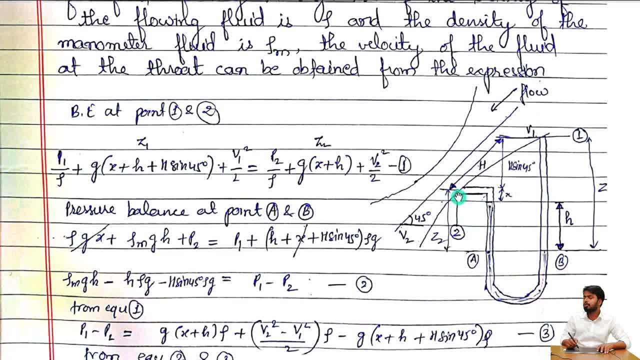 is v1 square by 2,. similarly, we have to write the Bernoulli equation for this point. then we took h plus x, so g x plus h. okay, gz2 plus v2 square by 2, so v2 square by 2, now 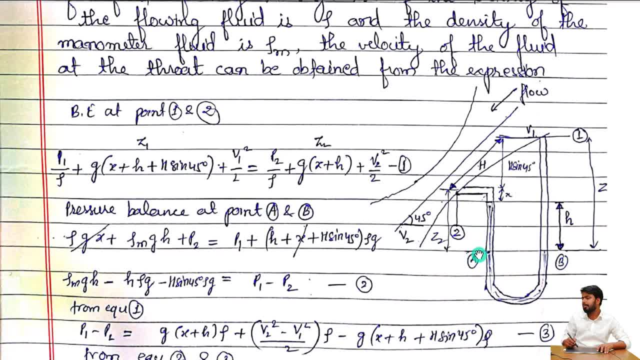 what to do. balance at point A and B. now, A and B is the manometric, where we have said earlier that there is no density variation on which we have to draw a data line. here you draw it, here you do the pressure balance. then what is rho? into g, into x? then what is this rho? 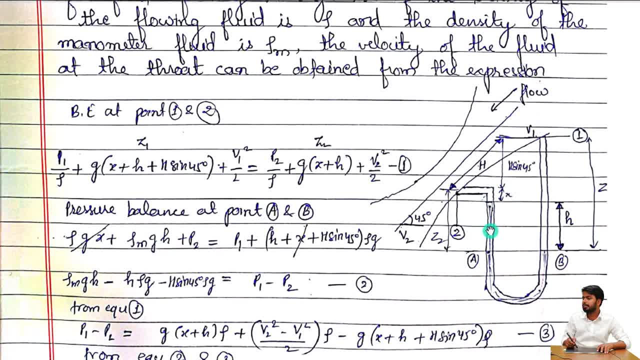 into g into x, plus rho m into g into h. then what is the manometric fluid of its density, rho m into g into h? here the pressure is p2,. similarly, here also p1 plus h plus x plus h, sin 45 degree has come into rho, into g. similarly we have to find the height here 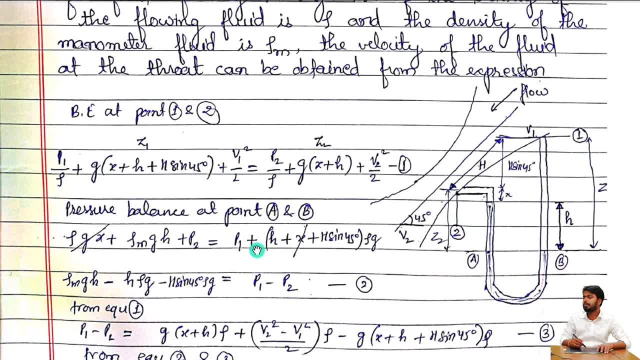 in the manometer. we have to find the pressure. how much is the height of this? p1 plus rho g is z1, the value of z1 is given. this is it now what we have to do? if you equate,